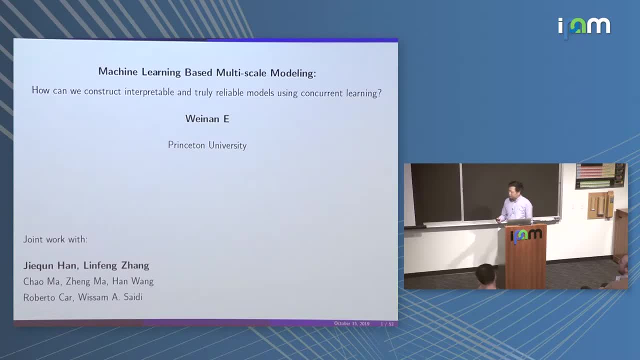 is how do we construct interpretable and truly reliable models, And you can see there is a lot of activity going on If you look at the poster. there's lots of things happening, So it's now fairly easy, not such a difficult task. Students can do it almost automatically. 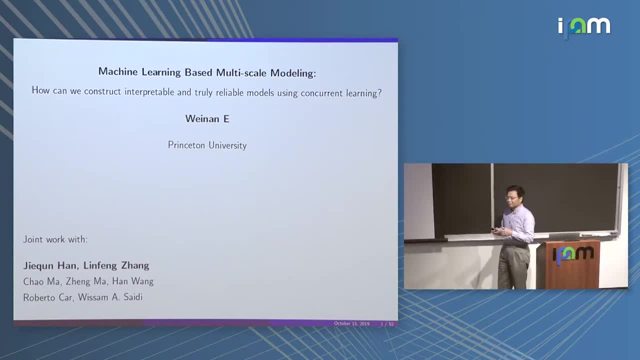 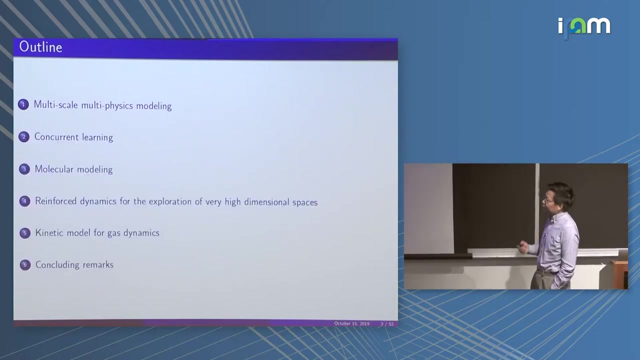 to get a bunch of data and fit the data very nicely with neural networks or something like that. But then what? So? what are we doing about this? What does that mean? So let me begin. So this is my outline, But let me begin with. let me wait for Stan to sit down. I was very 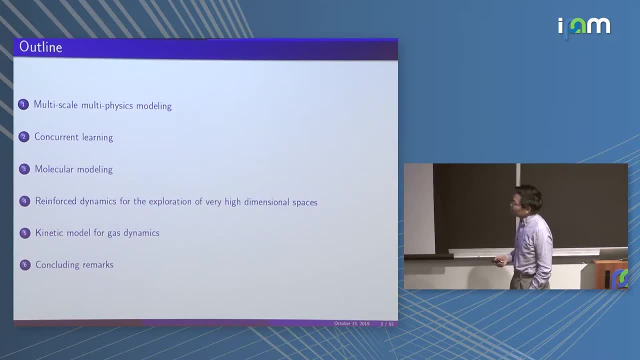 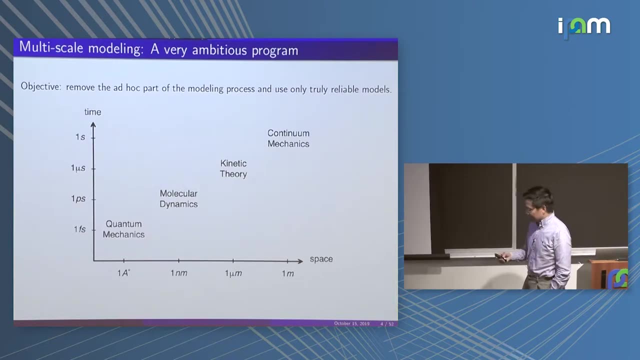 disappointed he wasn't going to come OK, so let me start with multiscale modeling. This is something that I devoted at least 20 years on. So the idea is that we, as an applied math person, as a math person, we 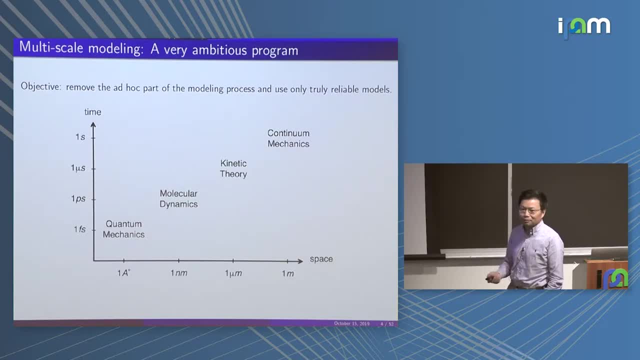 don't like this ad hoc stuff in the modeling process, For example, turbulence models, very dirty, unreliable, I mean I'm putting it very valid But in some sense there's a lot of work that has gone into it and has done, produced lots of progress. But on the 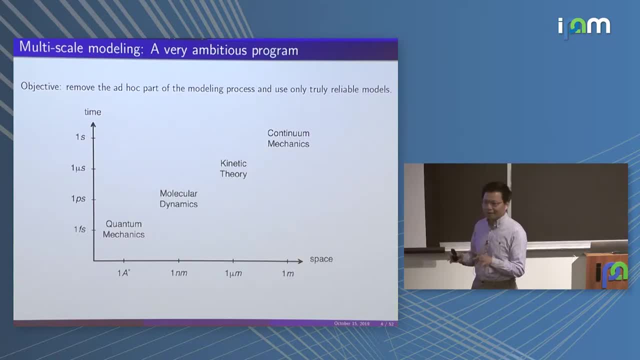 other hand, from our viewpoint, it's not clean. There's lots of ad hoc stuff. You have to rely on experience tuning a lot of stuff. So we don't like that And we want to do pre-supported modeling, new ad hoc stuff and accurate, reliable models. 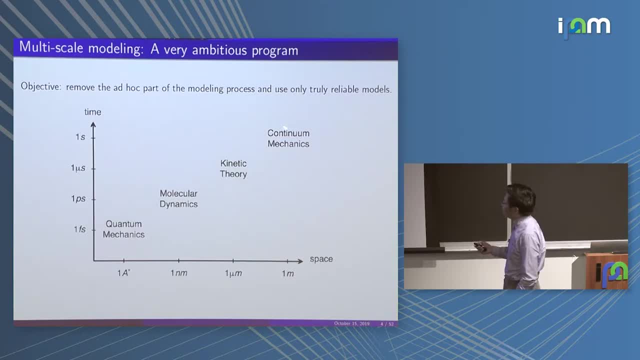 So that's the idea And the motivation for doing multiscale modeling, And typically we're interested in large-scale systems And in here, if you look at a plasticity problem, there's not very many reliable models. But on the other hand we all know quantum mechanics, at least the Schrodinger equations. 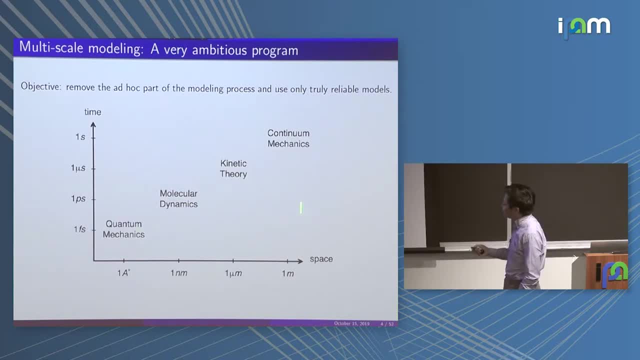 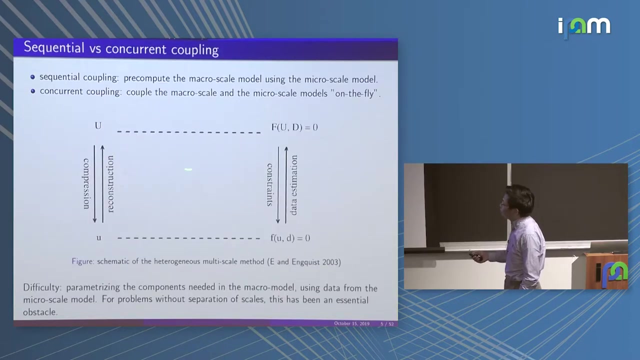 is truly reliable. So the idea is: can we produce models that would work on this scale but using, relying purely on information, that models at this scale? You can do that, either that our non-рос goes up. we can do this kind of empirical modeling by doing it now. 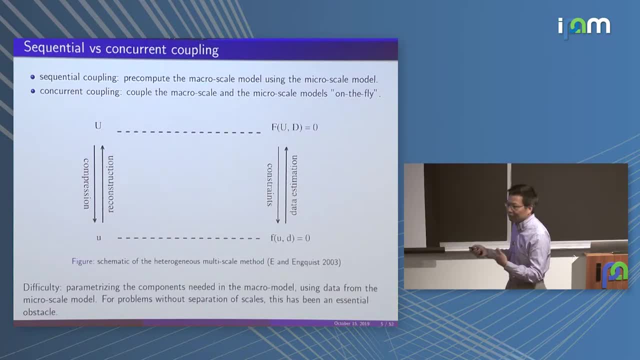 There are two ways to do it. You can either do a sequential modeling, which is they try to precomputing model, and then it's just as good as PDE, your Navier-Stokes equation at a macro scale. That's pre-computing, that's called sequential multiscale modeling. And 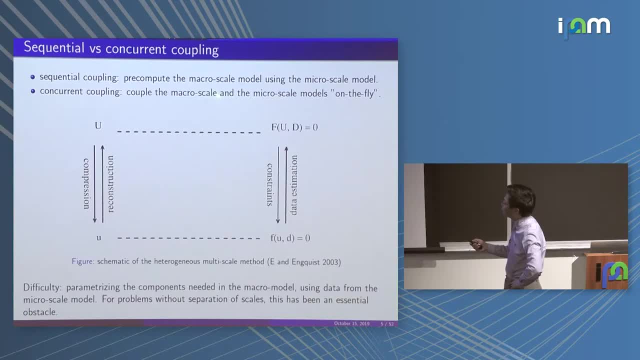 the other way to do it is to do it on the fly. So this is about getting a new model. This's about in an algorithm that it allows you to couple the macro scale system- over here of interest- with microscale models on the fly. 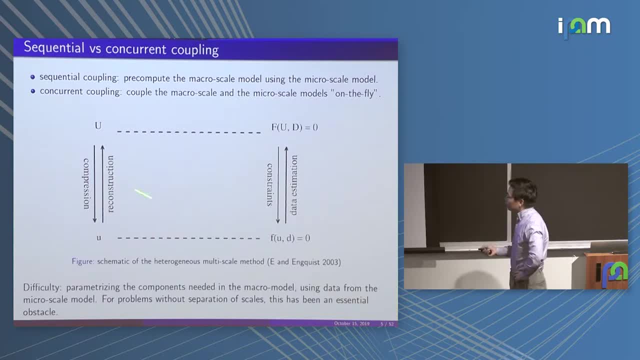 So this is called concurrent coupling. So the typical example: you know really you want to work at macroscale, You have a model which you don't really know. There's lots of components in this model, For example Reynolds stress. you don't really know. 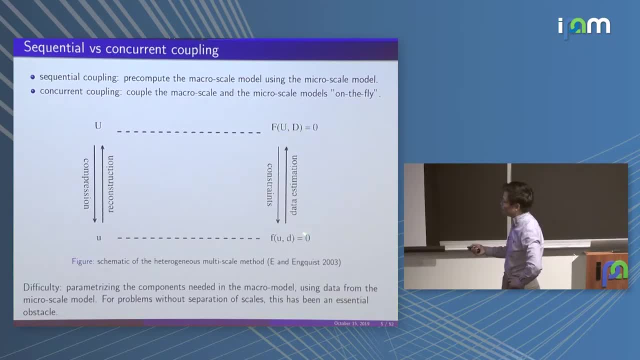 And you're supposed to compute that from some sort of microscale model. So this is schematic for what is called heterogeneous multi-scale method that Bjorn Anquist and I developed. But essentially the same spirit goes to other multi-scale algorithms, For example quasi-continuum equation three. 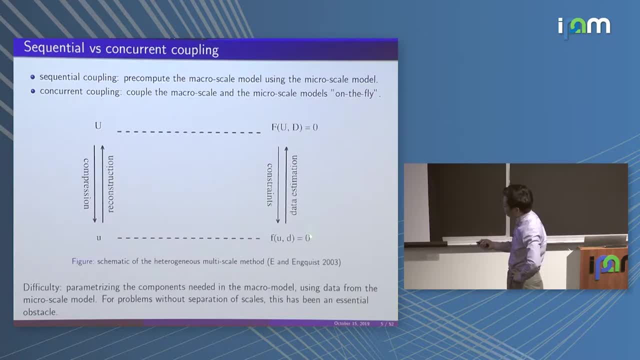 that Jan has developed. A key component here is this data estimation. You're missing some part of data. Reynolds stress You're supposed to estimate that data from the microscale scale model, And this is: you can do this if there are only like five. 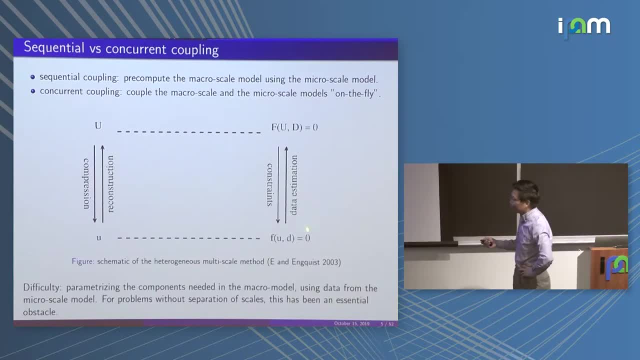 maybe five is already too big, but two or three degrees you can do this estimation. But if there are millions of degrees of freedom you need to estimate, And this is particularly the case when there's no scale separation, like turbulence. then you don't know how to do it. 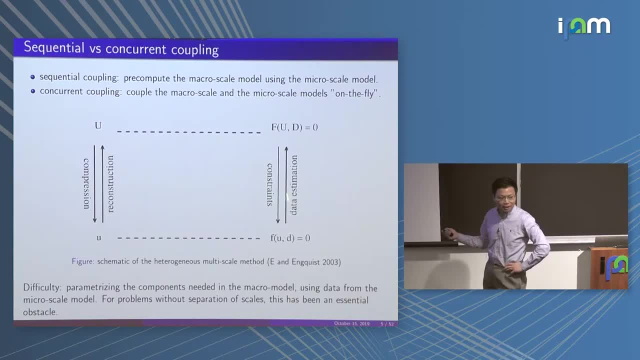 This was the obstacle, starting from the beginning. I already talked about this example, this difficulty, 20 years ago, And we didn't know for a long time we didn't know how to do that. And this is where the machine learning comes to the rescue. 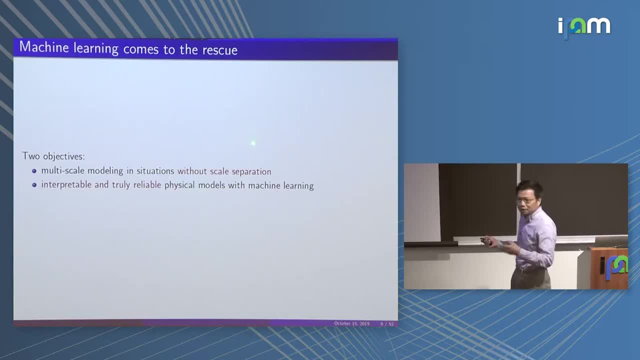 So now, with machine learning, our objective has changed, Namely, we want to develop multi-scale models- just the program I described- for situations where there's no scale, separation, turbulence. And we also want our model to be truly reliable, just like your Schrodinger equation. 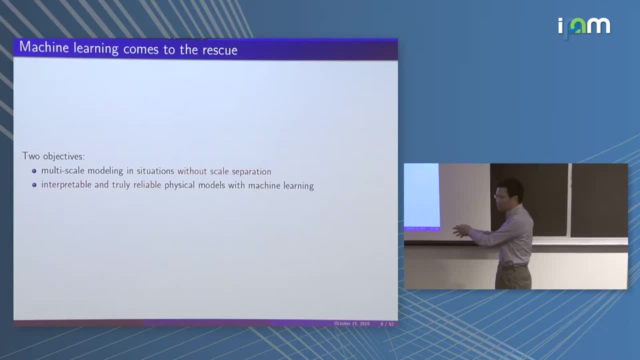 It shouldn't be just you know, it works only for your little data you generated, but it should be like you know new physical Navier-Stokes or Schrodinger equation. So this is what we want to do And let's see how far we can go with this. 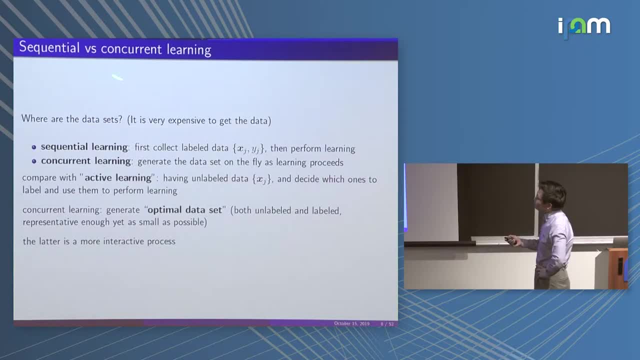 Thank you. So first I want to put up the notion of sequential versus a concurrent learning. I was just talking about sequential versus concurrent multi-scale modeling. So here I want to say that there are two situations of interest. One is the usual situation where you get your data first. 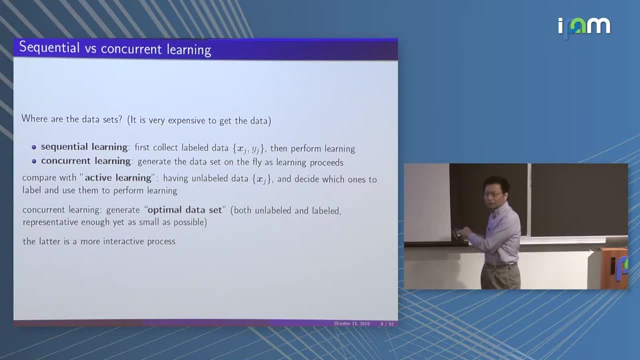 and then you use the data to do some model, to do some machine learning, And this is typically the case in artificial intelligence. image processing, computer vision, the data and preparing the data is already a huge amount of work. ImageNet is a good example. 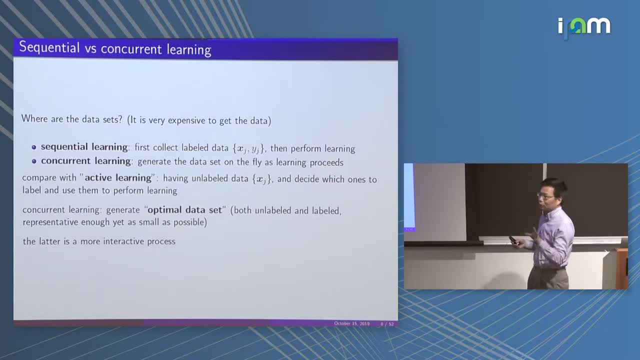 And then, with the data, you do some learning. So this I call sequential, because you first do data and then do learning. And the other scenario is that you generate the data on the fly as learning proceeds. In the beginning, as it starts, there's no data. 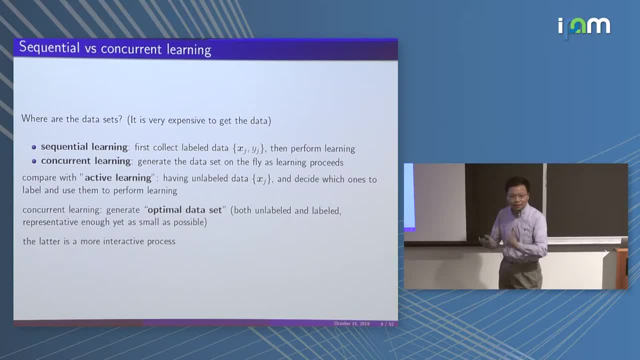 So you generate data and then you do the modeling, so interactively. So this is the scenario that we'll be emphasizing, And I want to put out this because this is number one. this is a little bit different from what people in machine learning used to do. 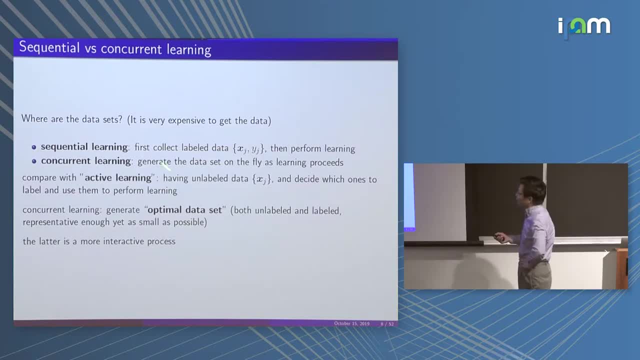 Number two, that there's a lot of more interesting questions. that happens here, And this is particularly from a mathematical viewpoint. there are more interesting questions. I want to compare this with active learning. So in a way, you would say that sequential learning is that you have both the data and 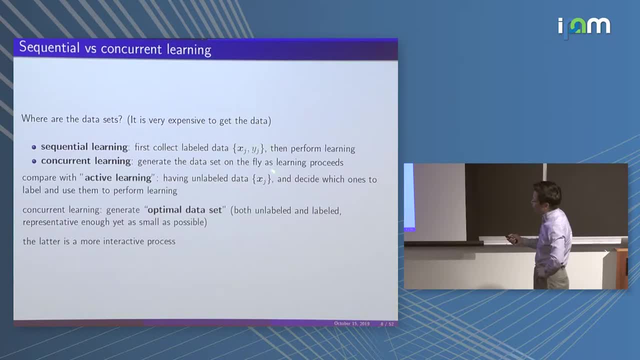 the label beforehand. Active learning is that you have the own label, You put it apart And then you decide from these unlabeled data which ones you're supposed to label and then do the learning. So this is what is called active learning. 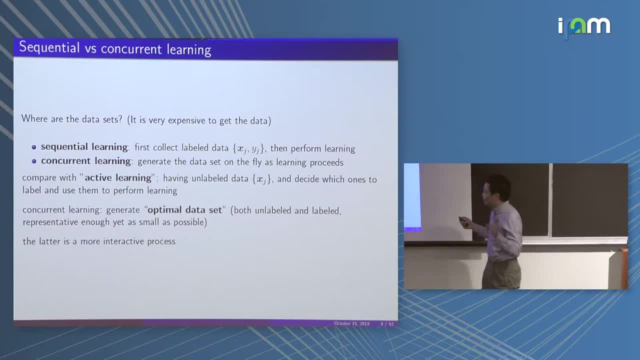 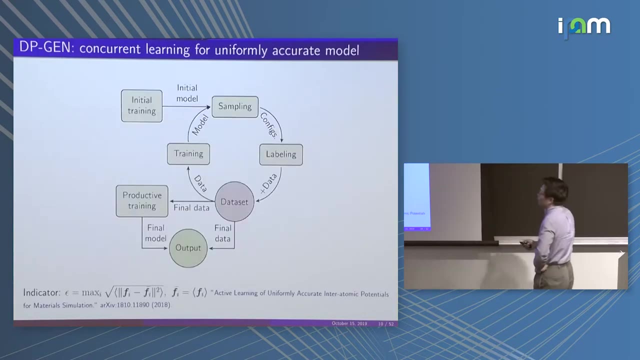 So concurrent learning is that you don't have anything to start with nothing, And generating these guys- not just the label, but also the data itself- is expensive. So you want to generate optimal data, So this is a much more interactive process. 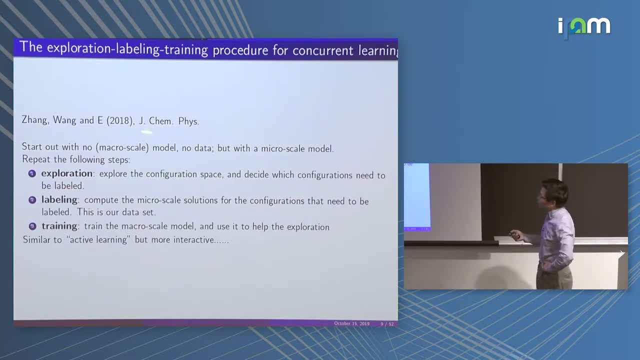 So procedure to do that. So this is A procedure that we proposed in last year. By the way, I would say, if you look at the literature, there are spirits of this everywhere. It's not like this is completely new, But we decided to put down this procedure, namely, you would start out with no data. 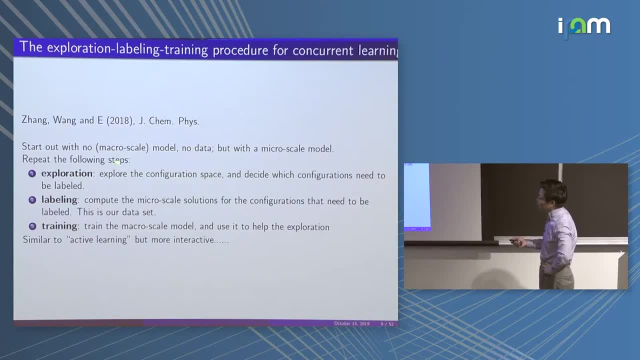 no model, no data, nothing. And then you first explore- You would explore the configuration space or state space that you're interested in, and then decide which one of these configurations need to be labeled, And then you do the labeling and then you do the training. 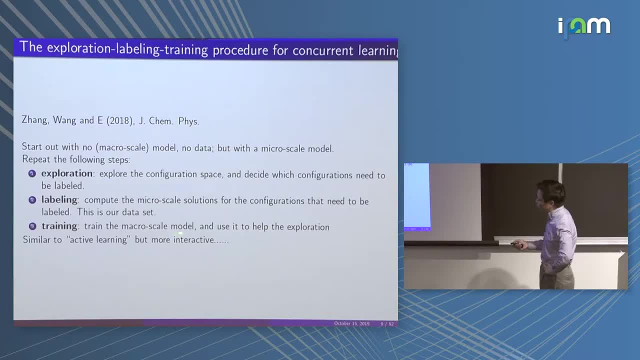 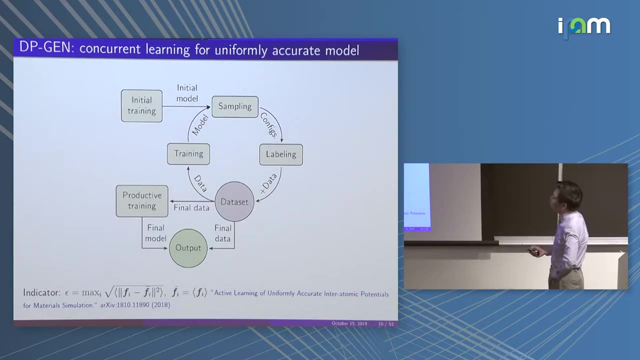 Now this sounds like the usual thing to do, but the important part is that this exploration is intact with the model that you have trained, So we'll see how to do that. This is a little more interactive than active learning, So this is the cycle. 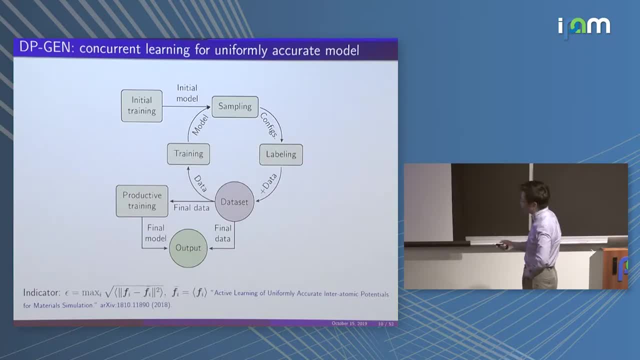 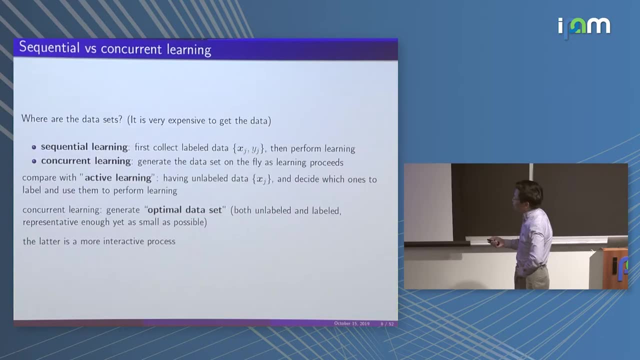 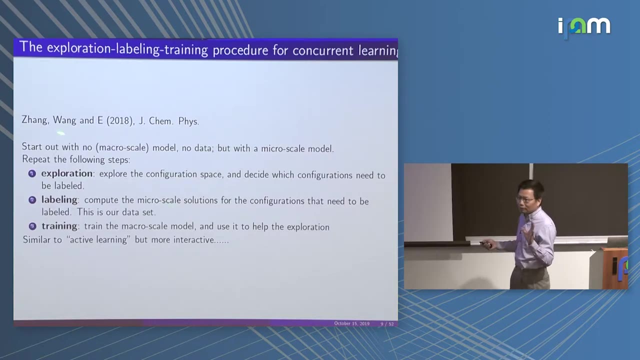 So you have, You have. Okay, This is what I just said. Now, let me just mention that. So there are several questions. First, Well, this is very sensitive, So the first question is: how do we explore? The second question is: how do we decide which configuration that needs to be labeled? 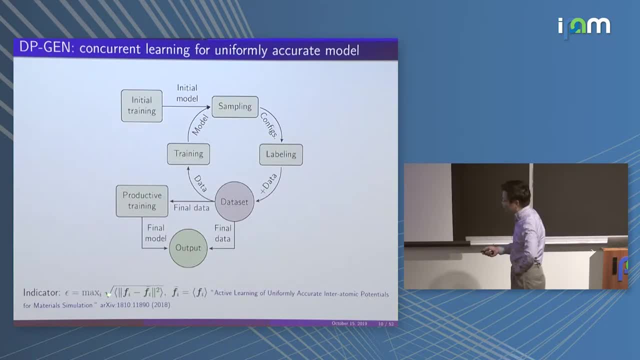 So let me now mention a trick that's used- I would say that's used- in active learning, which is the following little trick, Namely. So here the idea is that You should label the data where there's not enough data. 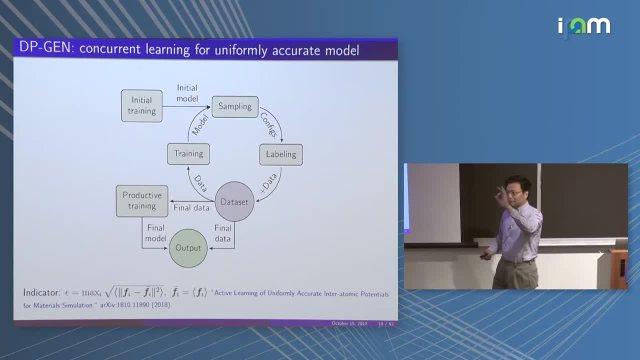 So if you see a little new configuration, you decide whether you should label the data. Label the data means that you need to do a microscopic physics computation, For example. you need to do quantum mechanics computation of that configuration. So that's very expensive. 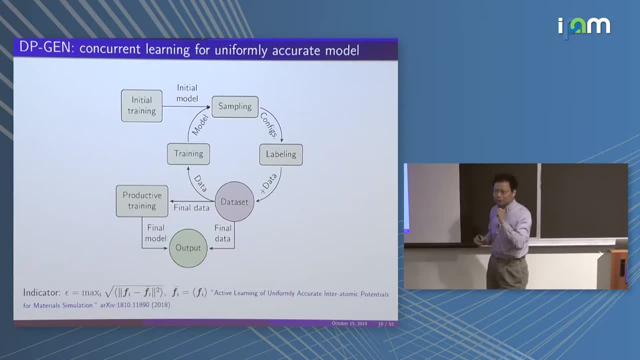 Okay, And you? How do you decide whether you should label this new configuration? Well, the principle is that you should label it when there's not enough data. If there's not enough data, then the model that you already have would not be accurate. 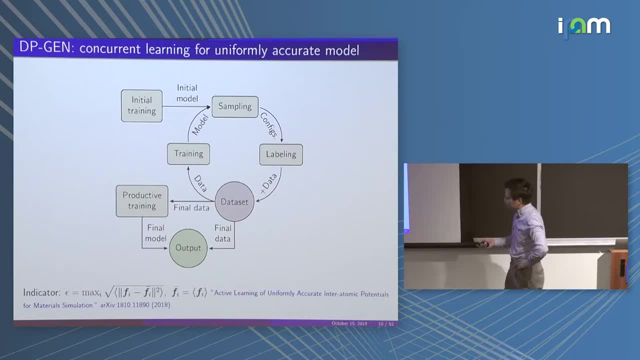 enough. Okay, So if you generate, If you train an ensemble of models- An ensemble means like four or five models- And if there's already enough data and your model is already accurate enough, all these models would predict the same thing for this new configuration. 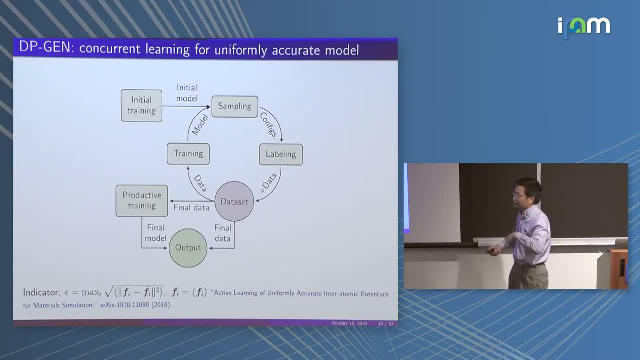 So if the variance between the predictions are big, Okay, Okay, Okay, That means there's not enough accuracy, not enough data, So then you should label that data. So this is a simple trick that people in active learning use and we adopt here. 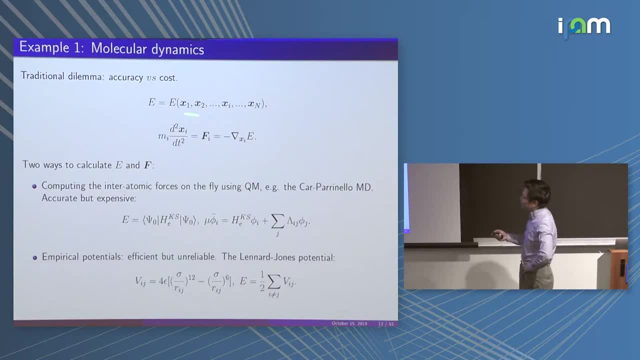 So let me give you some examples now. The first is molecular dynamics. Molecular dynamics: we want to study the dynamics of a system of atoms. So this could be a big molecule, or it could be a material. and by solving Newton's equation, 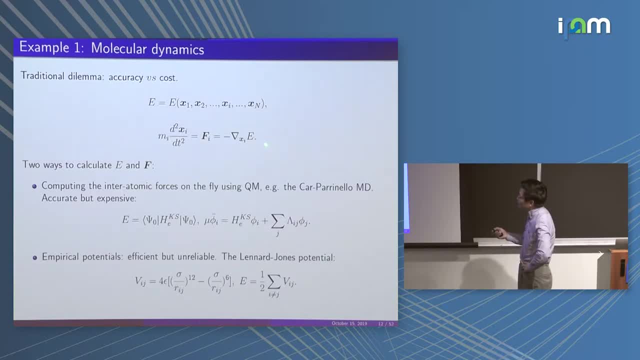 for the nuclei. So this is simple enough. The difficulty here? Okay, Okay, Okay. So you get the force. The force is given by a potential, So this will be the potential energy surface, And that's a function of all the positions of all the atoms that are present. 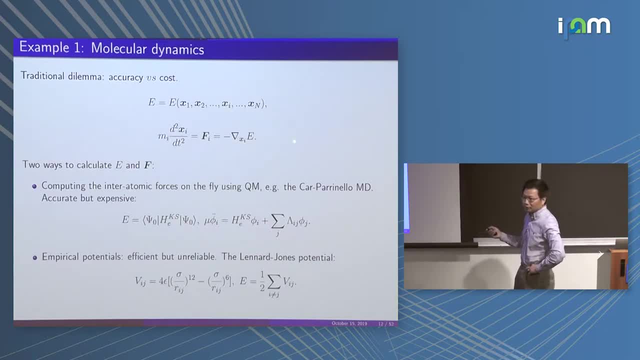 So if you have a million atoms, this would be a function with three million variables, And that's truly a large, dimensional, high dimensional function. So traditionally there are two ways to do it. One is developed by my collaborator, Roberto Carr in Pernal. 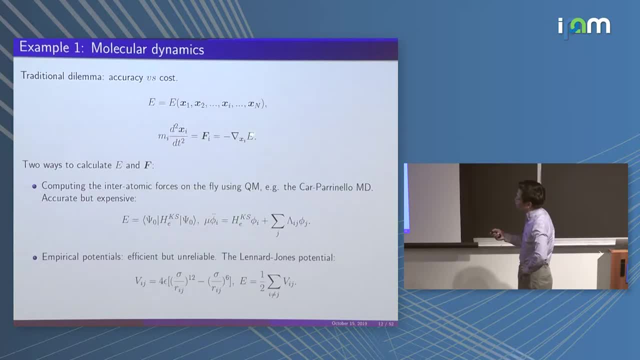 And that's to do, You know, To compute these forces on the fly, and couple that by coupling with quantum mechanics, usually density functional theory. So this is actually one of the most impressive concurred multi-scale modeling examples actually. So this is great, except that this is very expensive. 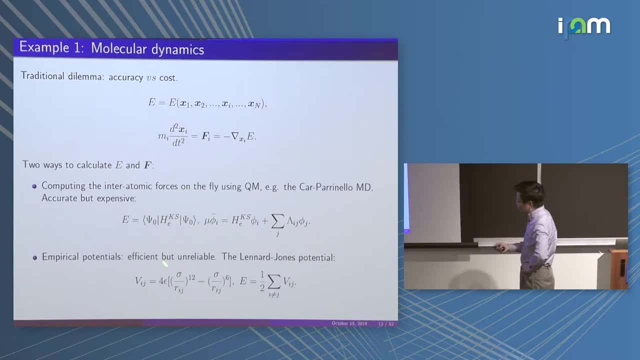 So you can't handle 100 atoms. The other extreme is that forget about quantum mechanics, let's just try to cook up a potential- you know empirical potential- that should model our system. For example, this is the well-known Leonard-Jones potential. 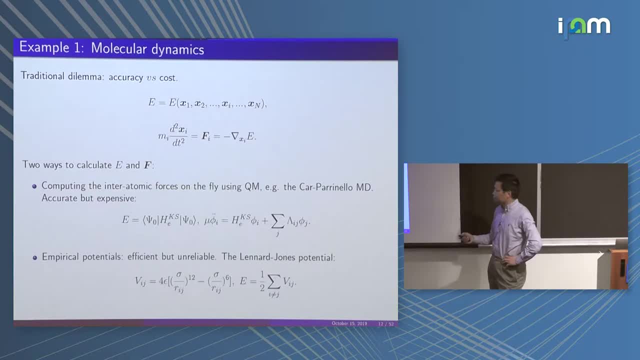 but there are much more complicated potentials: EAM, Tursov-Brenner, all that kind of stuff. So this is very efficient, much more efficient than this, but then it's not very reliable. So this is where you need to do a lot of tricks. 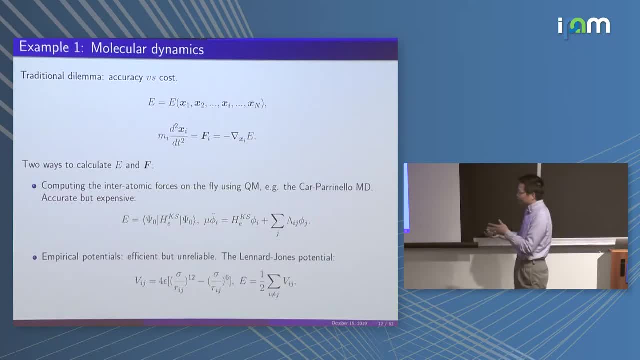 and you call intuition or you experience whatever. but in the end they're still not very reliable, particularly considering the fact that the data that goes into these models are very limited. So now the new: with machine learning we have a new paradigm, which is to say, 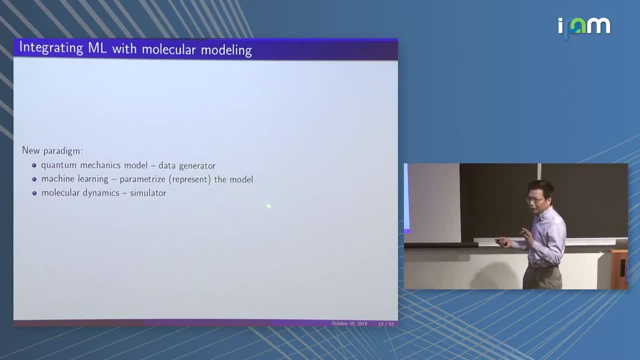 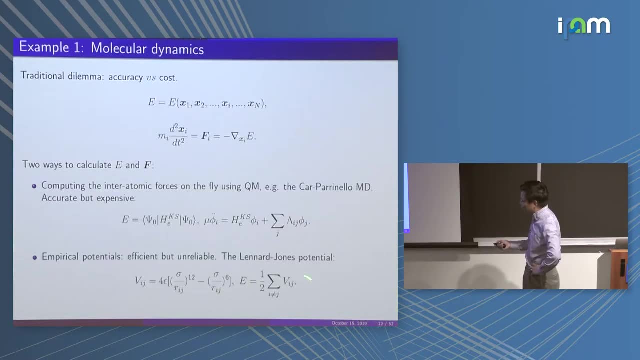 well, quantum mechanics just provides our data. We need to use quantum mechanics as a data generator. We use machine learning to parameterize the model, which would be in the spirit of this guy, and then we just submit it with a molecular dynamics. 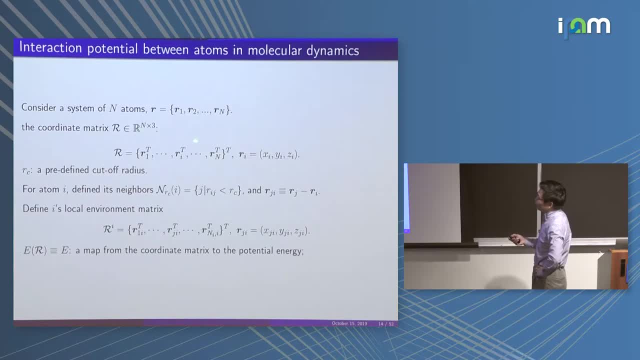 This is simple enough, Okay, so here is a little setup. We have these atoms, n atoms. Each one of these are the coordinates of each atom, and for each atom we define the little neighborhood. So RC is a cut-off radius that we specify beforehand. 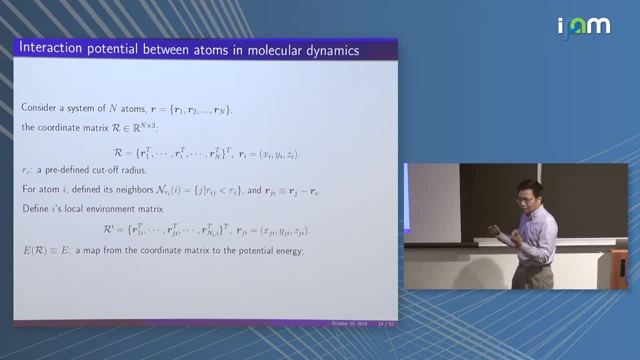 So for now, what I'm talking about is only useful when the long-range core interaction is not so important. So we're just working out the long-range part, but it's not published. So you think about this. this system only has reasonably short-range interactions. 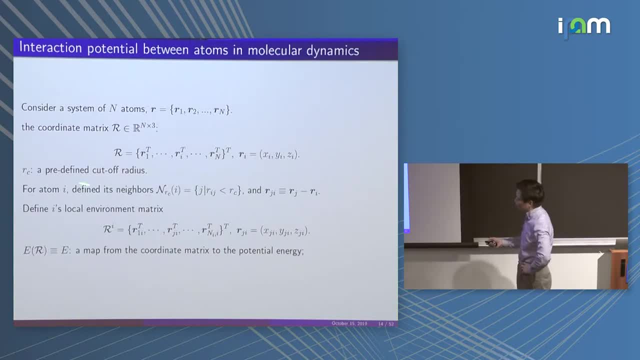 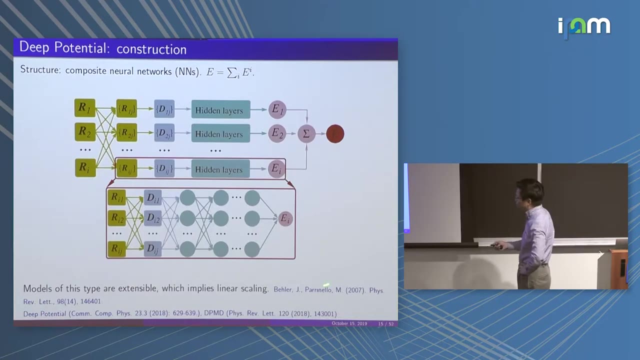 So then, everything the action is in the little neighborhood with the cut-off radius RC. Okay, and then for Each atom has its own little environment. So here is the network structure that was first proposed by Bella Pernello in 2007,. 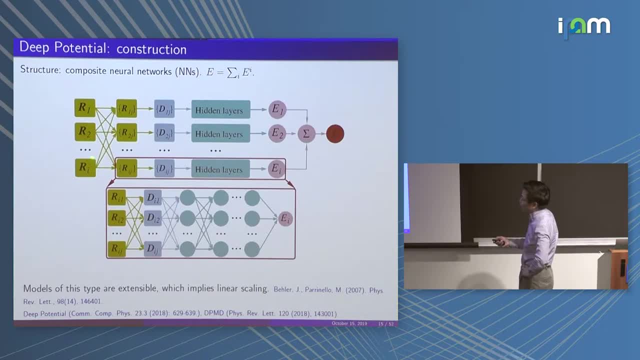 when neural networks were not that popular. So you have these items, atoms. Each one of these atoms has a subneural network And for each atom, the subneural network, the input, are the coordinates of the neighbors for that atom. 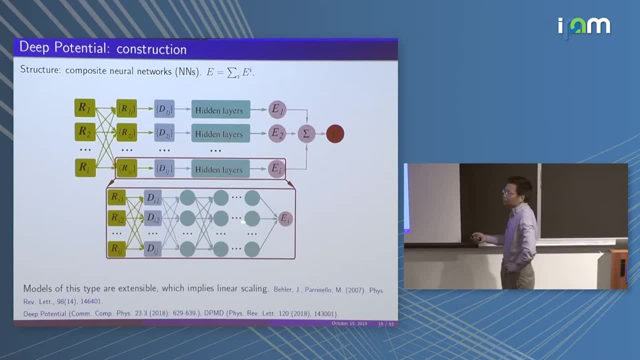 And then you're supposed to do some fitting- you know neural network, whatever stuff- in the end come up with the accurate energy. So this is the basic network structure. It's by having this network structure it enforces that this system is additive. 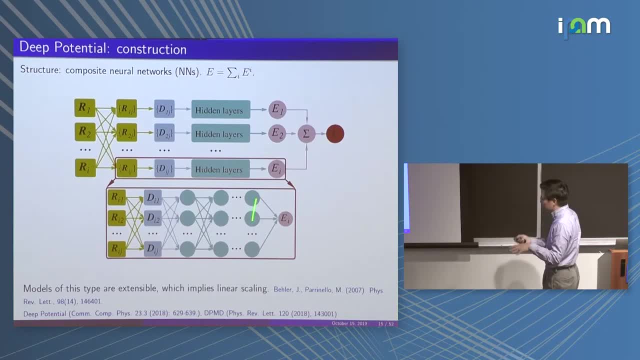 So linear scanning, If you have more atoms, you just produce. I'm just asking if those are shared. Yeah, the neighbors are shared. yeah, The neural networks. Well, if the same atom is shared, If the same atom is shared, but it's. 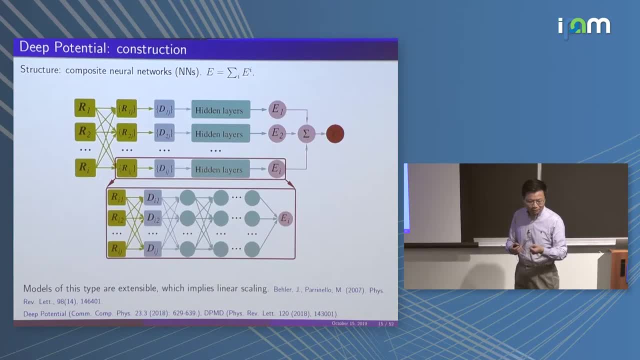 Okay, shared, but if it's different it's not right. So there's a little bit of difference between oxygen atom and hydrogen atom. Oh, so there's atom-specific function. Right, right, Okay, But I think 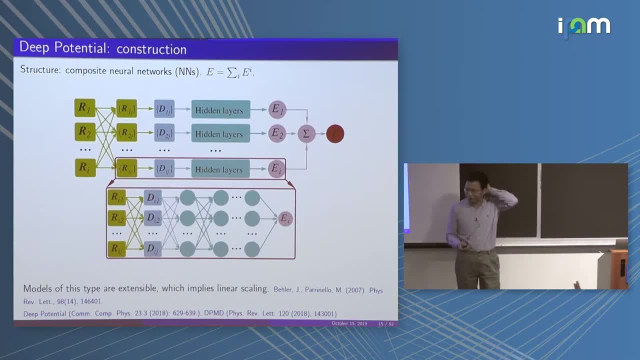 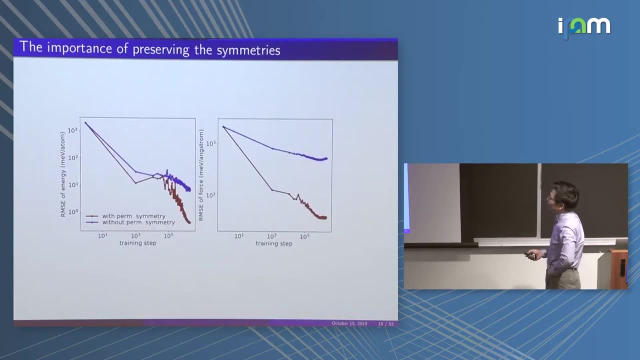 You don't even necessarily know right, You can give like the feature. I think in the end this is shared. Yeah, I'm not that 100% sure now Okay. So the first point I want to make is that 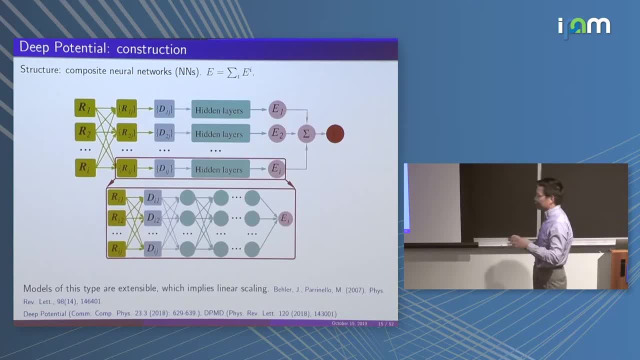 preserving symmetry is very important Here. besides the usual translation and rotational symmetry, there's a new symmetry which is permutational symmetry. Namely, if you have two copper atoms, you label this one and label this two, and vice versa. it's the same system. 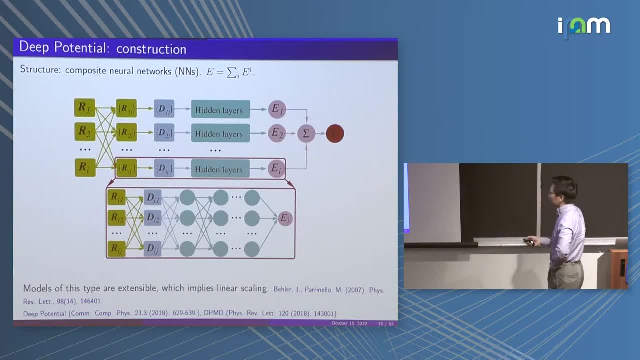 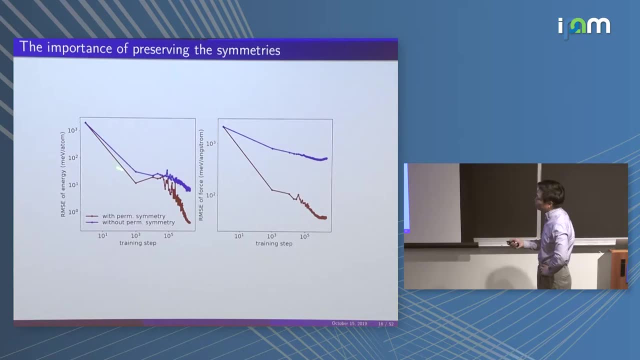 So things do not change. And that's indeed So. that's permutation symmetry between the labeling. So that shows up very dramatically here. So if you don't impose permutation symmetry, the training error just doesn't go to zero, It flats out. 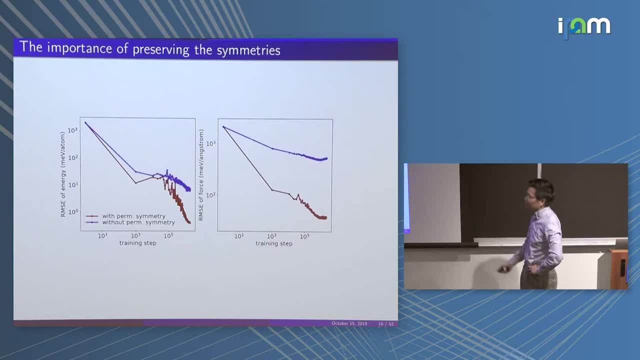 And if you impose permutation symmetry, then it goes down nicely, Okay. So another important point to make is that you should train with both energies and forces. If you just train with energy, that's also harder. So this is the first remark. 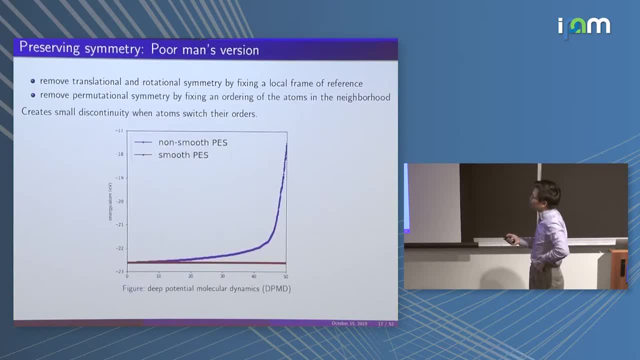 You should really put in permutation symmetry. The simplest way to put in permutation symmetry is to fix first of all: Well, there's more than permutation symmetry. There's translation, Translation, rotation and permutation. So for translation and rotation, you can fix that by imposing a local coordinate system. 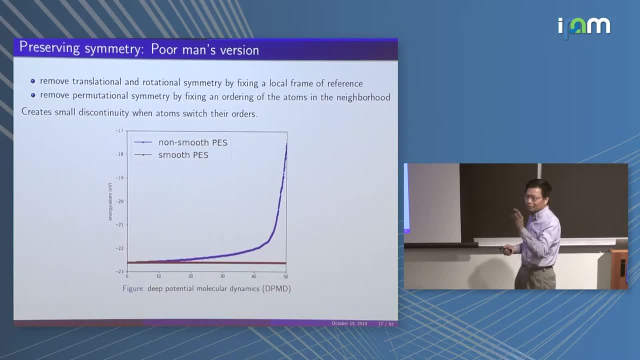 for each atom. You fix the atom you are looking at as the origin and then somehow define a frame. So that would fix the rotation and translation symmetry. For permutation symmetry, one way to do it is just to have a way to order them in the little neighborhood. 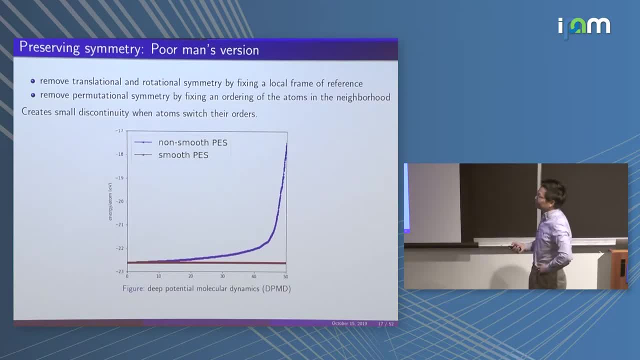 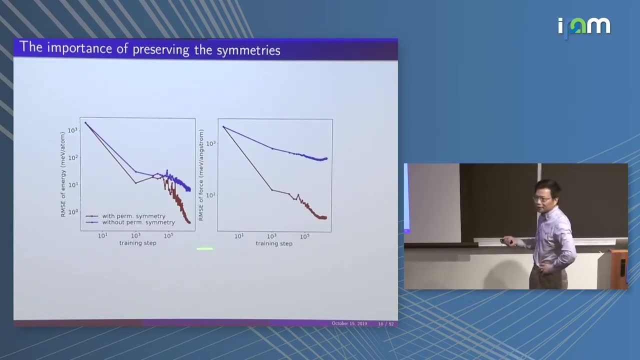 That's sort of a poor man's version of fixing the symmetries And that works out here. when you look at the training errors and the testing errors, that looks good, But when you put that into molecular dynamics and run for a long time. 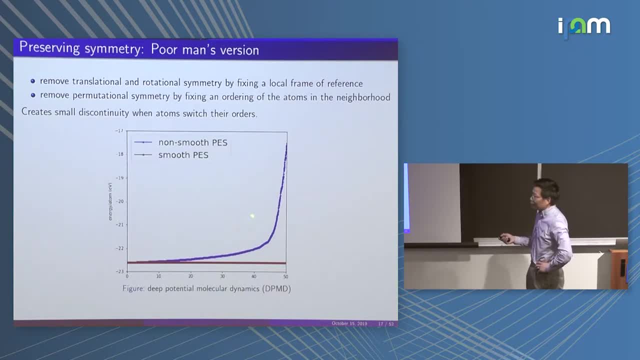 then you see a systematic drift of the energy. That's because in the process of labeling, ordering the atoms in the neighborhood, this is done by looking at the distance between the neighbor and the atom you're looking at, And suddenly the distance can change. 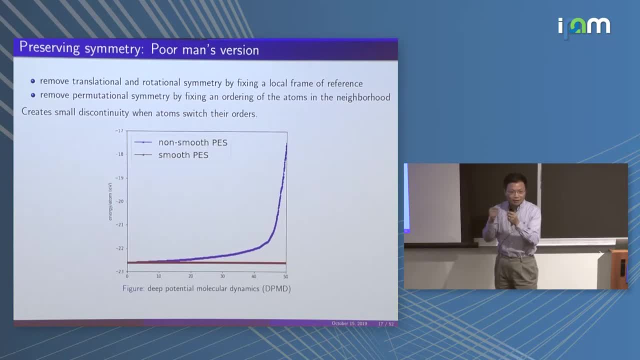 And that change changes the order suddenly. So that introduces a little discontinuity. That little discontinuity gives a little force, thermal force, into the system and causes the energy to drift up. That's not good. So really we have to enforce the symmetry in the right way. 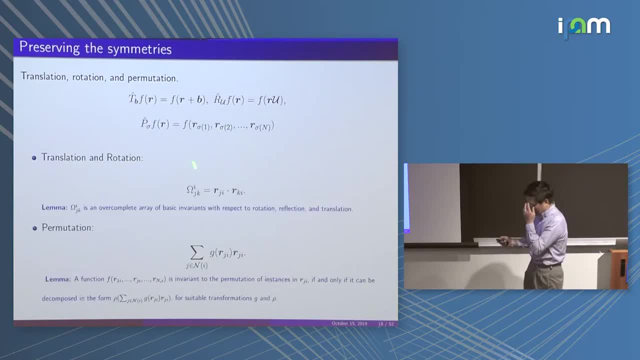 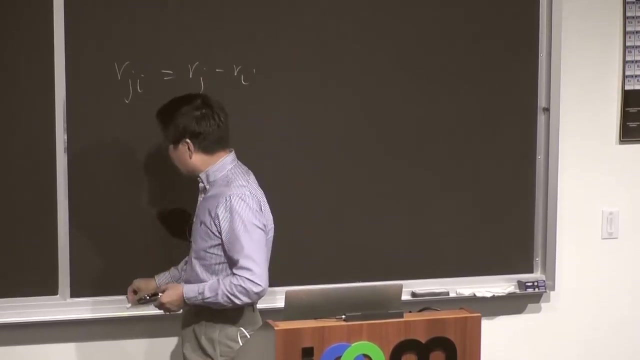 And the way to do it is the following. So first of all, these Rji, they are the Ri minus Rj, So these are the relative positions. So we're looking at the atom Ri, and Rj is another atom in the neighborhood. 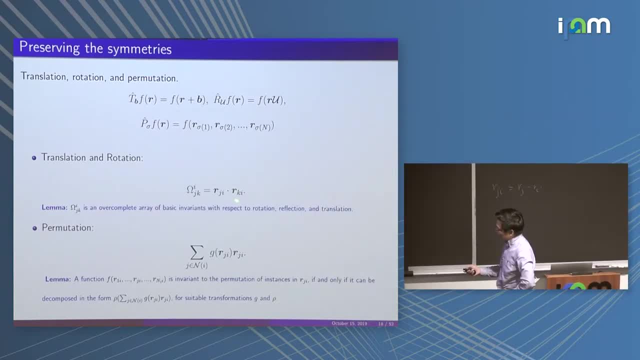 So if we look at these quantities, they're automatically translation and rotation invariant. And if you look at these quantities, they're automatically rotation invariant, So permutation invariant. So we're going to design a network that only uses the quantities of this type. 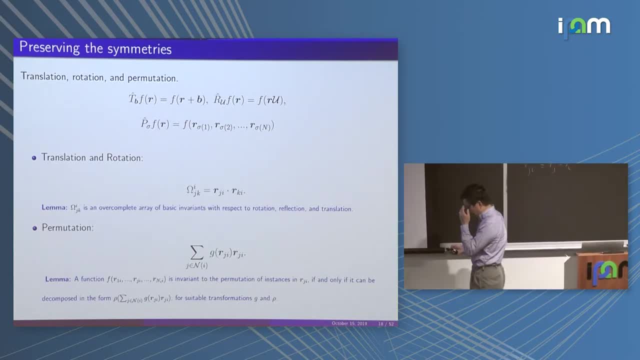 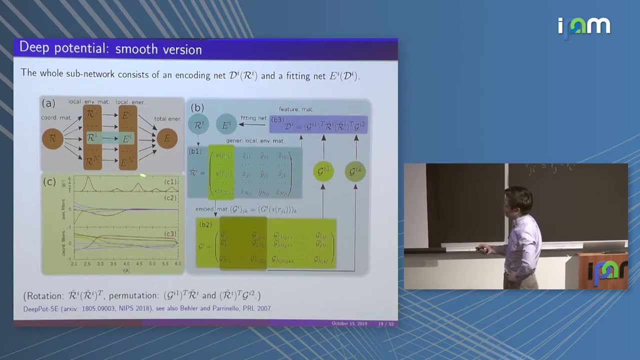 So automatically it has to be translation and rotation and permutation invariant. So here's what's happening. This is a very busy slide. So for each- I said for each- atom, there's a sub-network. for each atom, The input is just the neighbors. 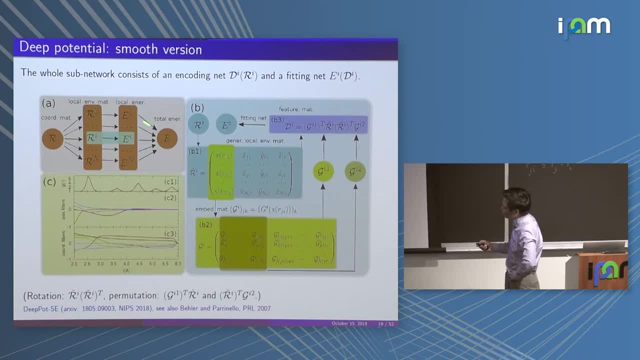 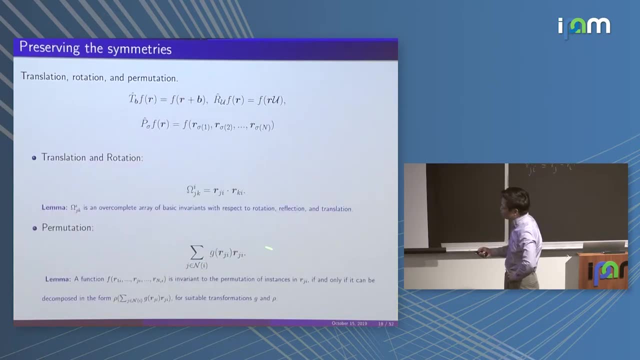 for that little atom. But each sub-network has two parts. One is the encoding part, one is the fitting part. The encoding part generates many, many functions of this type, of this quantity. So therefore the output of the encoding part are symmetry-preserving quantities. 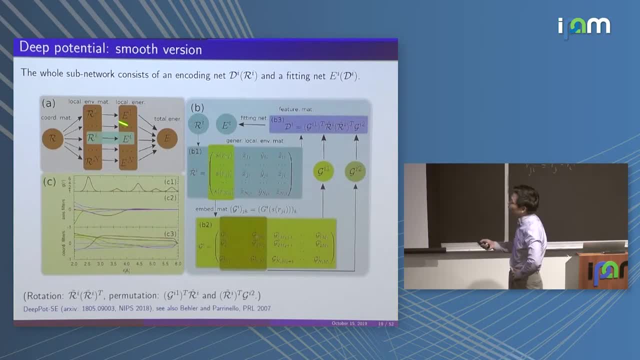 And we make sure that there's enough of those, And the fitting part is the neural network that fits the energy and the force. So that's what's going on in these sort of slides And, as a matter of fact, it seems that these filters. 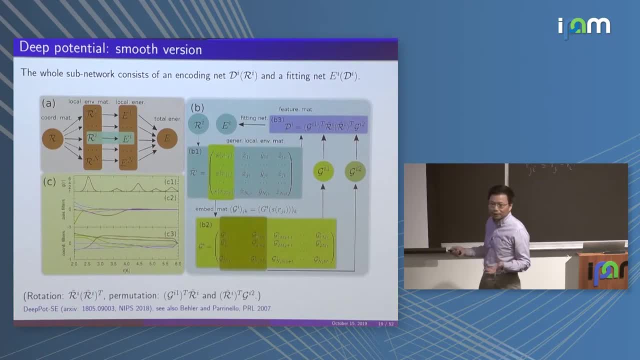 in the first encoding part seem to have some sort of interpretation, So I'm not going to talk about it too much here. But in a way this is a very smooth and it makes sure that all the symmetries are preserved. So this is the first part. 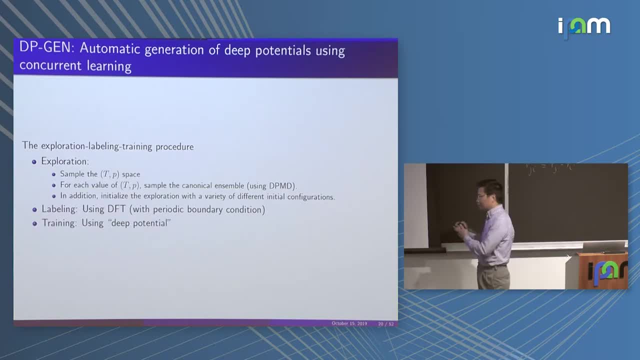 This part is like sequential learning: You give me the data, then I produce a neural network that fits the data. The second part is that. Can I have a quick question? Yes, It seems like you're suggesting the smooth version is energy-preserving. 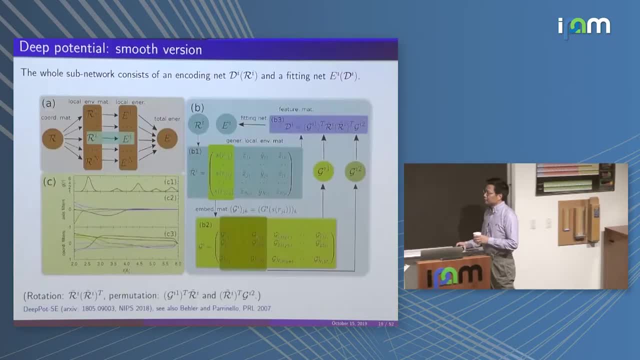 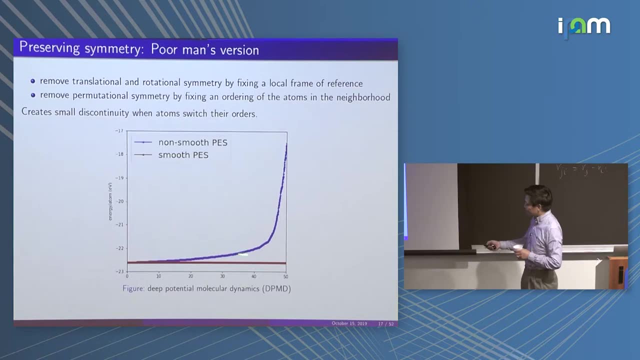 Is that somehow enforced or is that just? No, it's not reinforced. So this is the result. This is very sensitive. Got to give it a. This is the producer with the smooth version, But is that guaranteed to be energy-preserving? 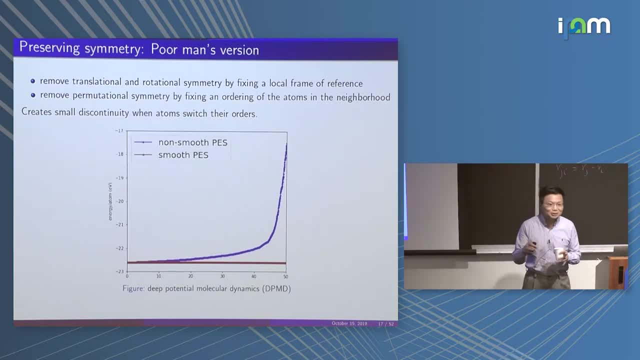 or it just happens to be energy-preserving. It happens to be energy-preserving by looking at it. There's no. If you want to prove it's energy-preserving, that depends on how your MD scheme looks like. It's not exactly energy-preserving. 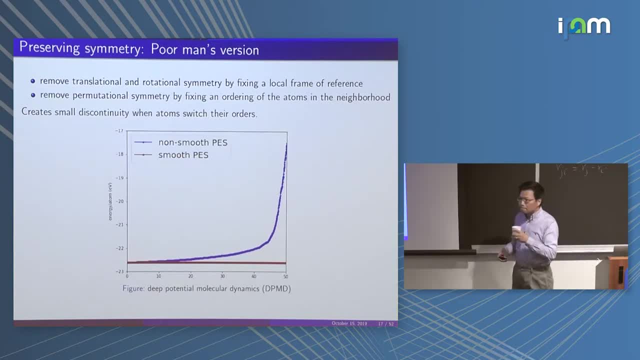 all that sort of stuff. Thanks, That's a follow-up question. When you say you're training both the energies and the forces, are you training them as separate learning targets or are you training them as the energy backdrop and the broad backdrop again? 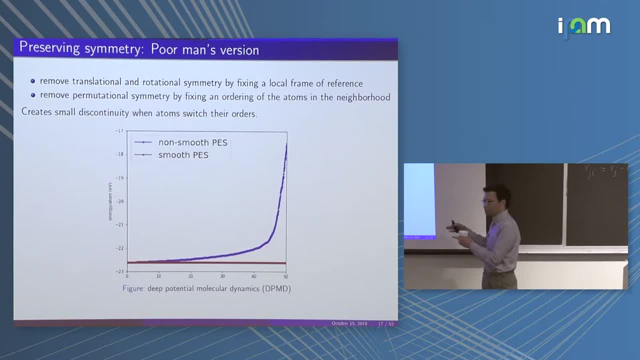 In the loss function there's a part that's energy and another part that's force, And these coefficients are tuned to adaptively as training goes on. So is the force computed as the gradient of the energy. Hm Is the force computed. 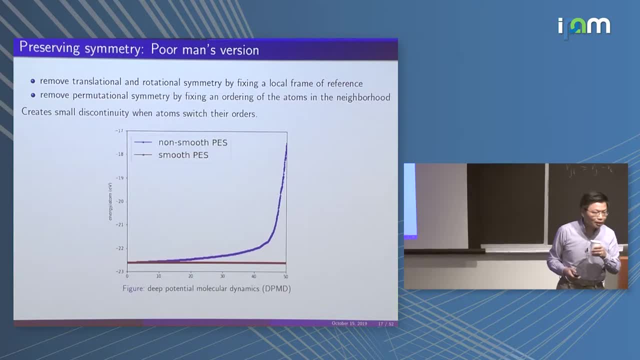 as the gradient of the energy. Yes, yes, Okay, so what if there's no data? You just, You want to do aluminum and there's no data. So here's the procedure. Here's what is concurrent coupling, Concurrent learning. 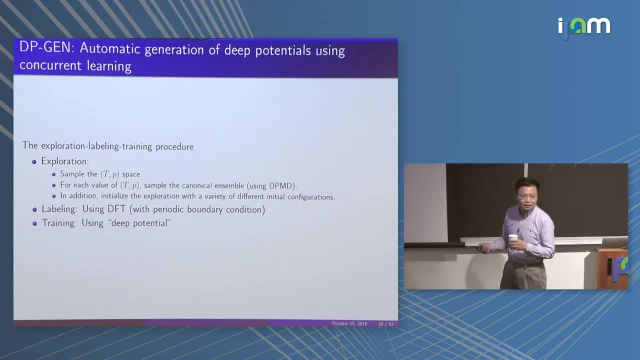 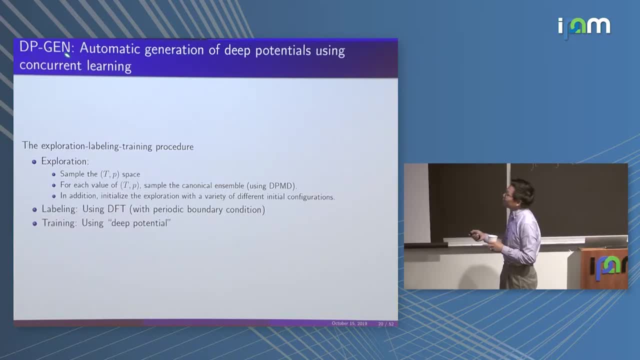 DeepJane, DeepJane, DeepJane, DeepJane, DeepJane. So this, So this is called Deep Potential Generator. So here is, following this procedure: exploration, labeling and training. So for exploration we sample. In this case we sample. 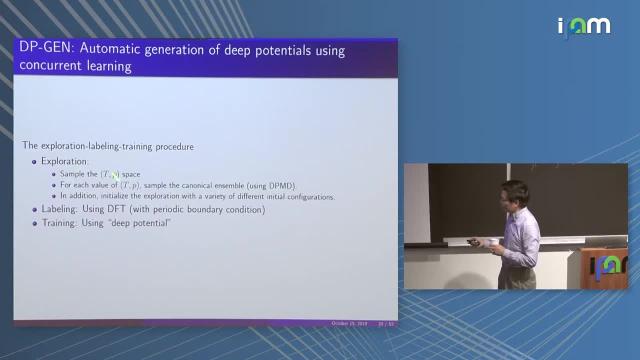 There are three components. The first is sampling the macroscopic thermodynamic variables space, And for each one of these variables you sample the canonical ensemble using the DeepMD, or we'll call it DeepMD It's- I think the name is made up. 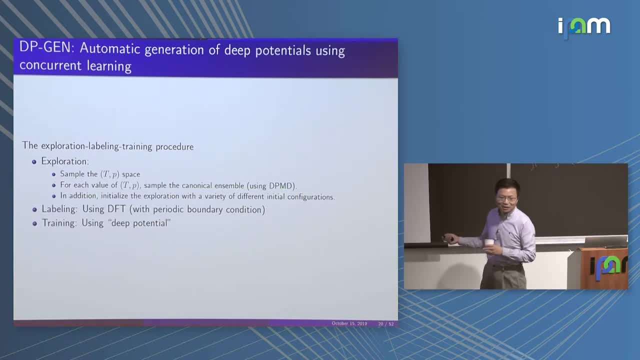 by Roberto Karr, because there's CPMD, there's DPMD. CPMD is the Carp Perinello Molecular Dynamics. So now it's DPMD- deep potential, deep potential, molecular dynamics, By the way, we call the potential deep potential. 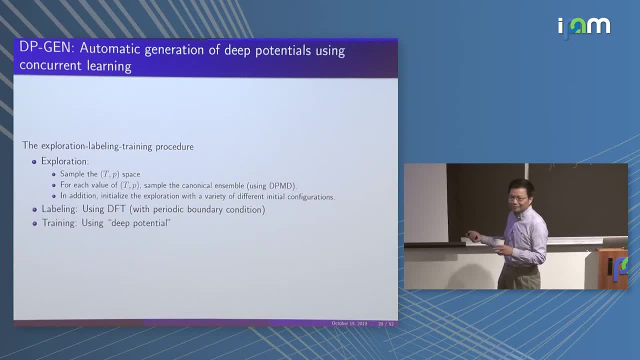 And this was like three years ago, when there's not so many deep things yet, but now everything's deep, so this looks a bit. anyway, that's life, And in addition, we also initialize the exploration with a variety of initial configurations. 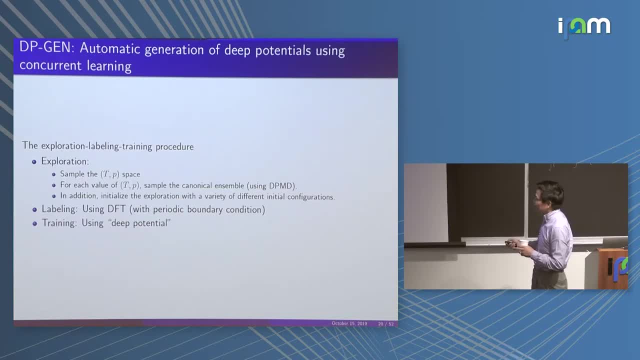 different crystal structures, hexagon or whatever cubic, that stuff. Labeling is just done using LASP DFT with periodic boundary condition, And the training is the deep potential I just described. Okay, so anyway, you do that. So now you don't need to generate the data first. 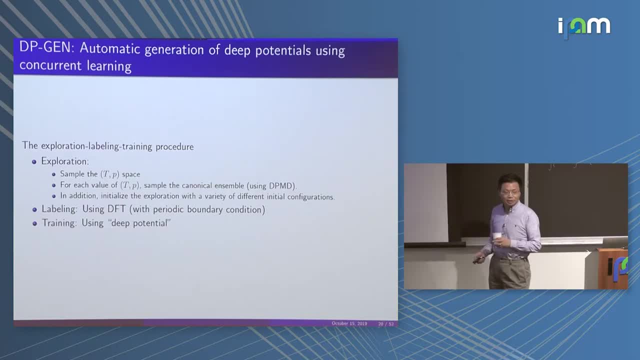 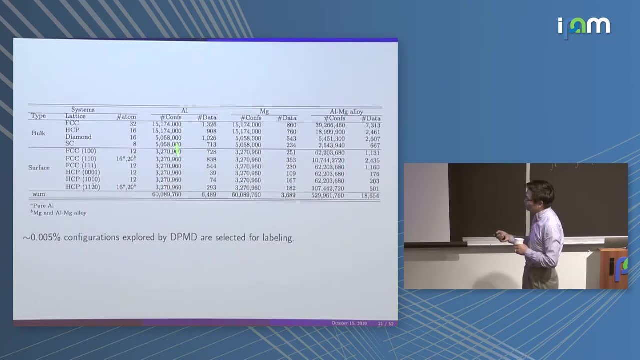 You just tell me whatever system you're interested in, this procedure will generate data for you, generate data and generate the model for you. And this just to show why how important this procedure is, exploration and this concurrent coupling is. So here are examples of aluminum, magnesium and the alloy. 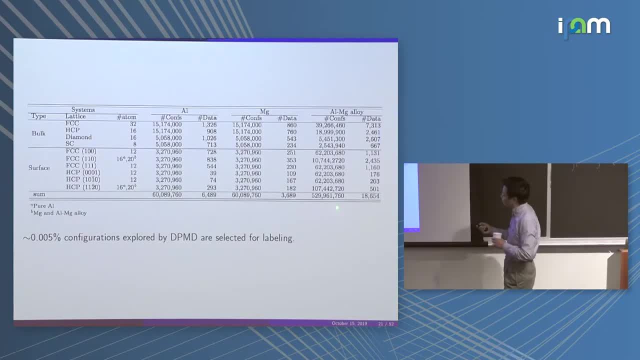 And you see, these are the numbers of configurations explored. For example, let's look at this: This: 500 million configurations explored and only this many were labeled. Very small percentage were labeled. Think about it if you want to label all those. 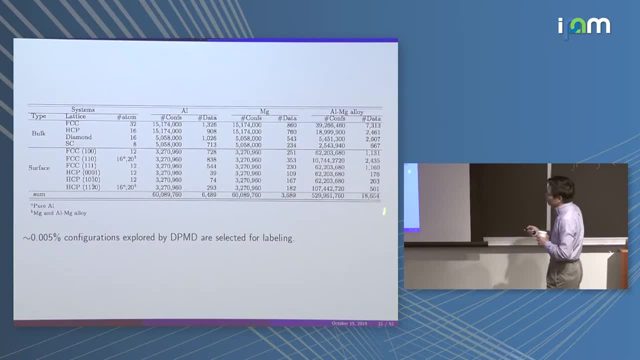 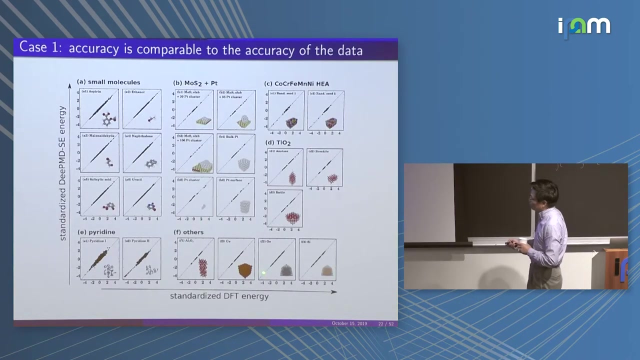 you know life would be much harder, But you only need those and the accuracy is just as good. So less than 0.0005% of labels of configurations need to be labeled. Show you some results. First of all, the potential itself is very accurate. 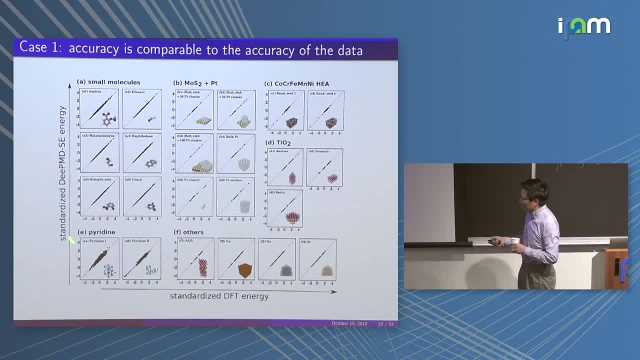 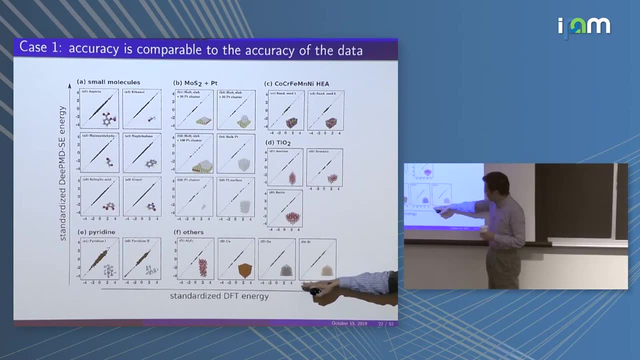 Basically, the accuracy is comparable to a DFT. So, for example, this big molecule, paradine. So you understand that if it's on the diagonal, it's accurate. This is like the DFT, This is the DFT, This is the predicted. so it's on a diagonal, it's accurate. 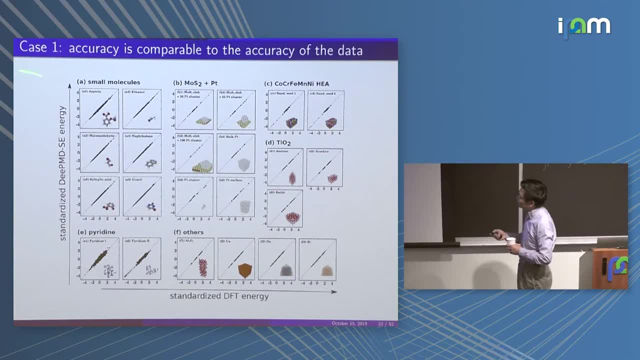 So, for example, these are small molecules. This is a high entropy alloy with five components. If you want to cook up, your empirical potential for this life will be very hard: Oxidides, surface materials and then big molecules. So the accuracy here is not so great because the DFT itself the accuracy is not so great. 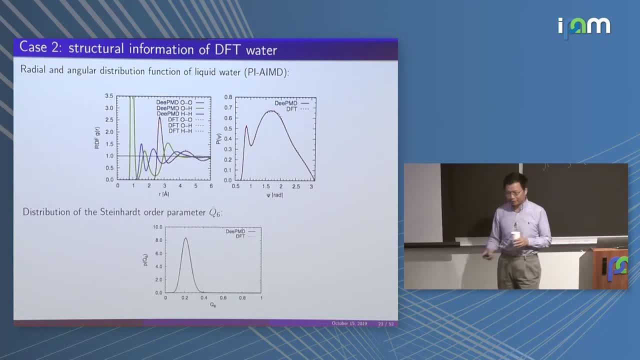 So basically it's comparable to DFT. So now we have to go to work on DFT. Secondly, if you look at statistical information, structural information, you don't see the difference. There are actually every curve. there are two curves. 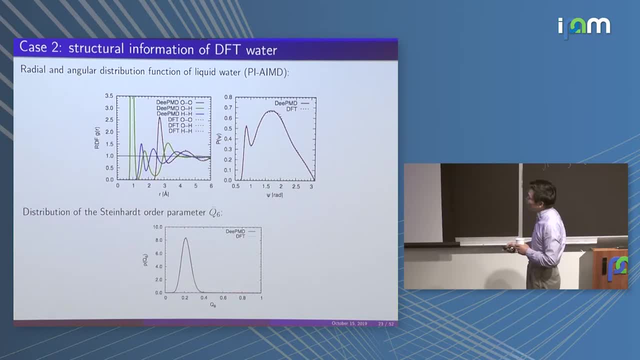 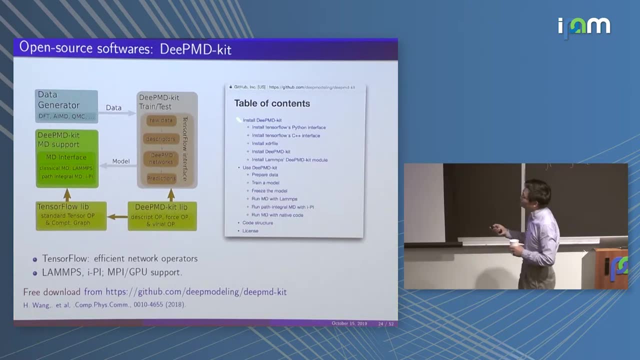 You don't see the difference between the DFT result and the DPMD result. So now we have generated software, open source software. So this is the deep potential. If you go to GitHub With DeepMind On the DeepModeling, there's a whole bunch of software. 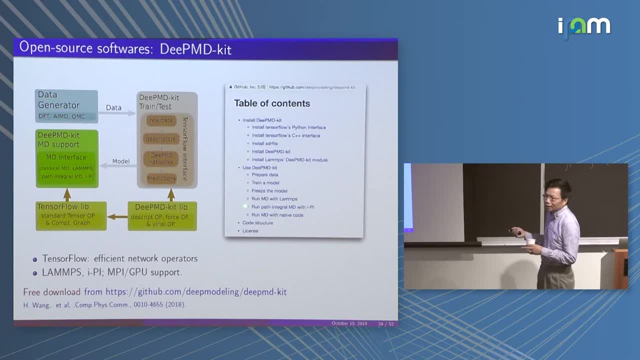 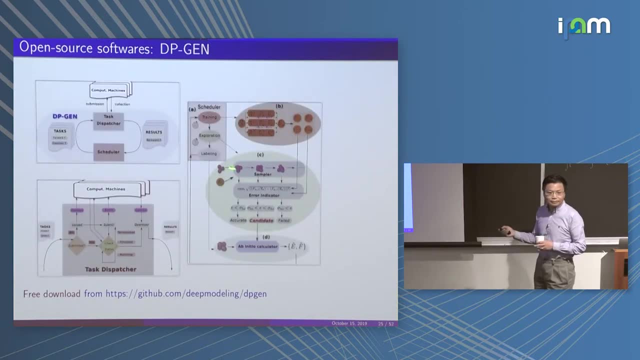 This is the deep potential. So in this case you need to supply the data and then it generates the potential for you. But now we have a version which generates the data. This is the concurrent learning. So you just have to tell the system what, tell the software what system you are interested. 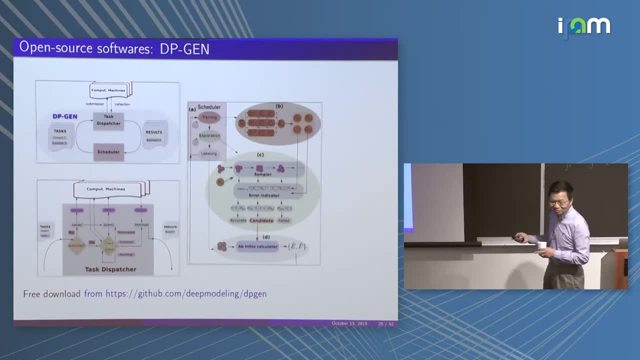 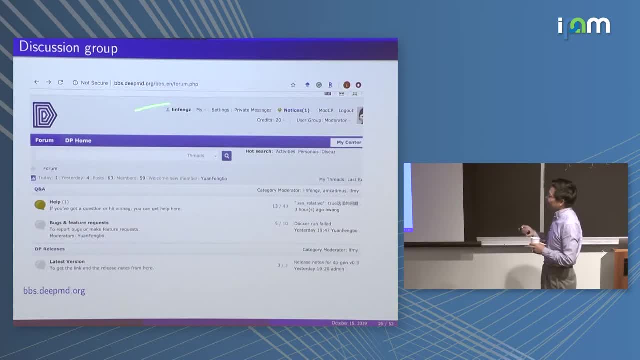 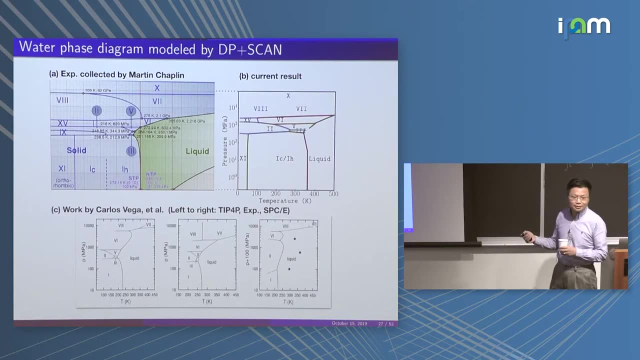 So there's a discussion group. That's very important because lots, you know, hundreds- of people are talking in this discussion group and they try to improve each other. I think this is the way to go, because it's it shouldn't be the case that each group has 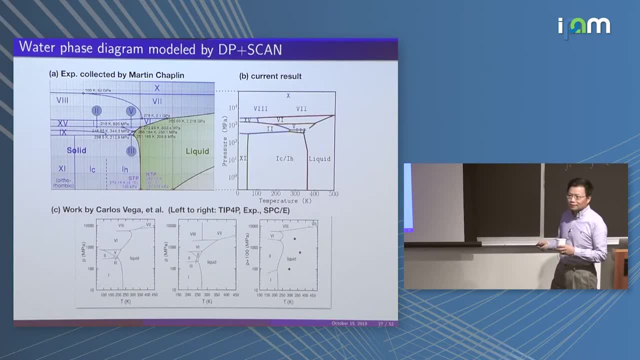 to do its own thing. So we just have this open source forum and everybody can contribute and everybody improves upon each other. So this is an application, Okay, Okay. So this is an application: Namely, we are developing what we think will be the universal model for water. 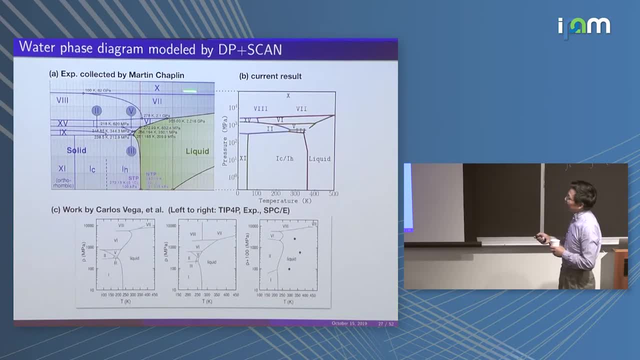 Water is a very difficult system, as you know, And experimental. this is the experiment. this is the phase diagram for water. It's supposed to have over 20 phases. I'm not an expert, Robertica is an expert. So it's supposed to have over 20 phases. 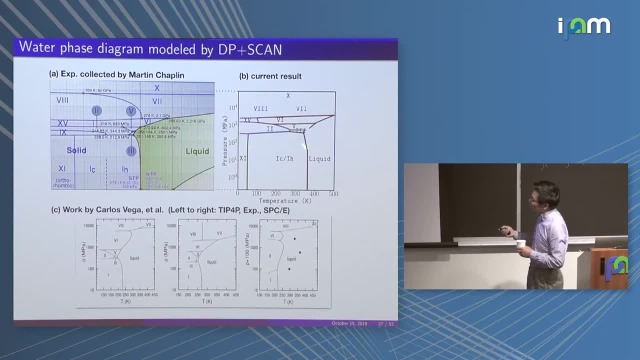 And the potential we have now generates. you know very close qualitative- at least qualitatively close- phase diagrams If you compare with what's done before TIP4P or SPCE. you know it's very, you know it's. 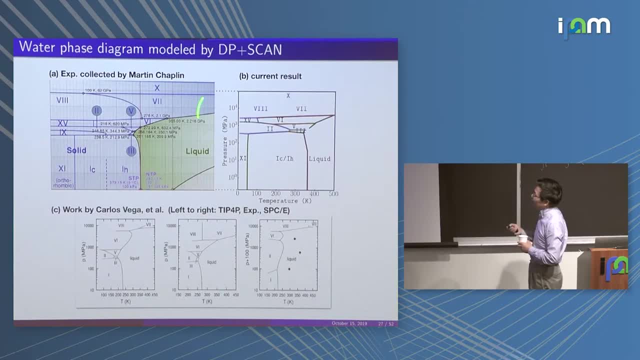 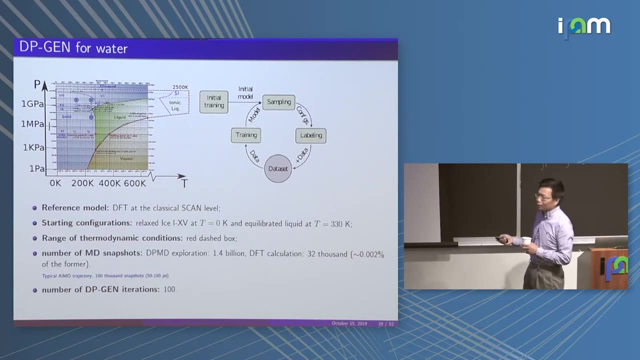 quite far from the experimental result. So now the phase diagram we produced. according to Robertica, it's the first time that one can produce qualitatively similar phase diagrams, And this is the details for generating the potential for the water. If anybody is into water, we can talk about it. 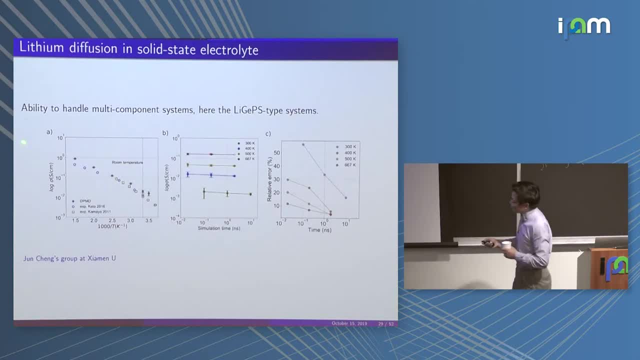 Well, actually I don't know much about it. So thank you. And this is the second example, which is the diffusion of lithium in the solid-state electrolyte. So this is battery. what is it? batteries, lithium-based batteries- right Nobel Prize. 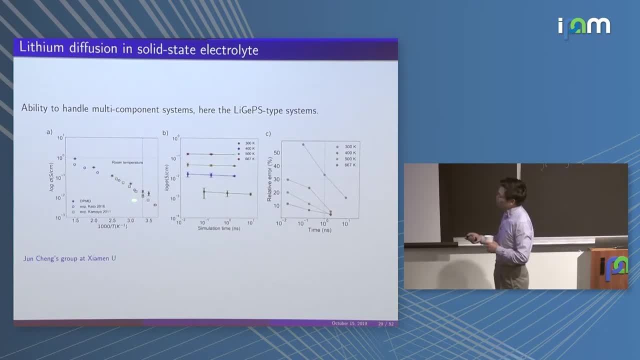 several days ago. So diffusion of lithium is the key thing for the solid-state electrolytes in between the cathodes And then before. people can only compute the diffusion coefficient at very high temperature and then try to extrapolate. So for the first time we can compute the diffusion coefficient at room temperature. 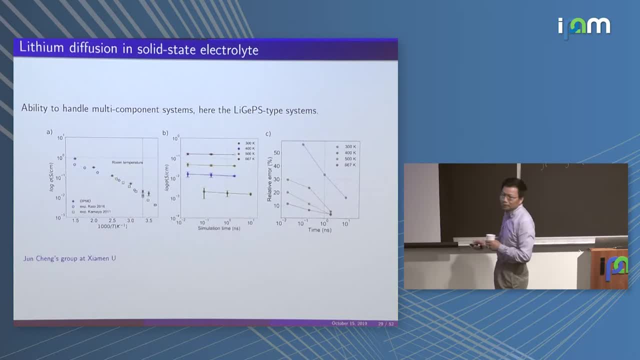 here and this compares reasonably well with experiments. That's because we have a system, we have a model which is as accurate as quantum mechanics, but it's much simpler than quantum mechanics. so we can use this model to compute very large systems for a long time. 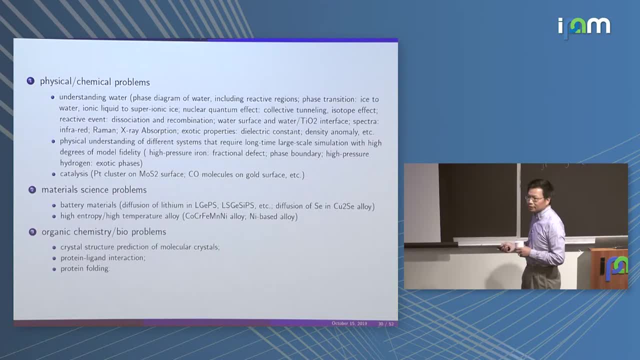 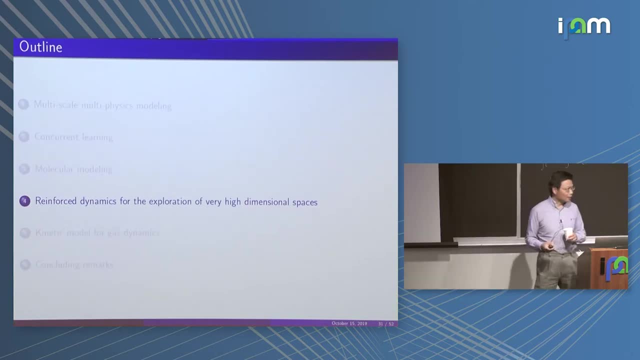 Okay, So there's a bunch of applications, many, many applications. that's going on. That's the first example. The second example I want to talk about, okay, the second example I want to talk about is how to? it's like protein folding. 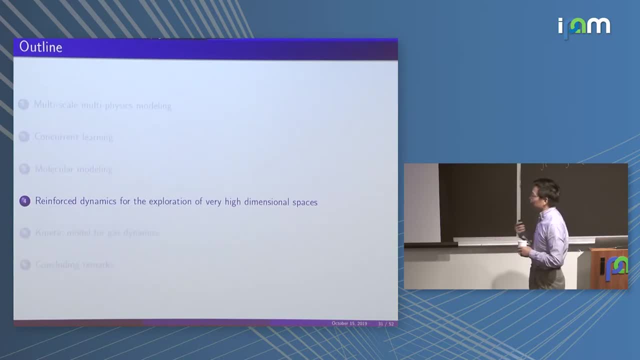 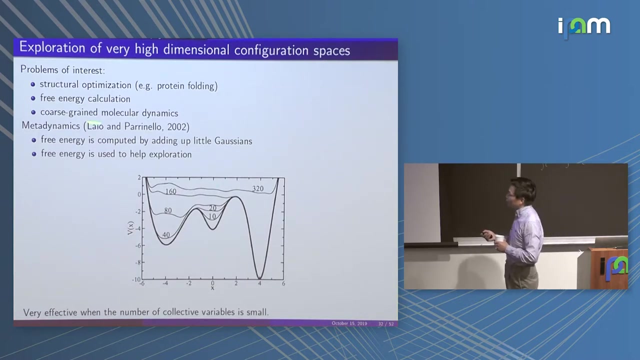 So here the thing would be protein folding, because you need to explore very high-dimensional surfaces, high-dimensional spaces, and you need to compute the free energy in that very high-dimensional surface. And a well-known example is called is a metadynamics developed by Lyall and Perinello. 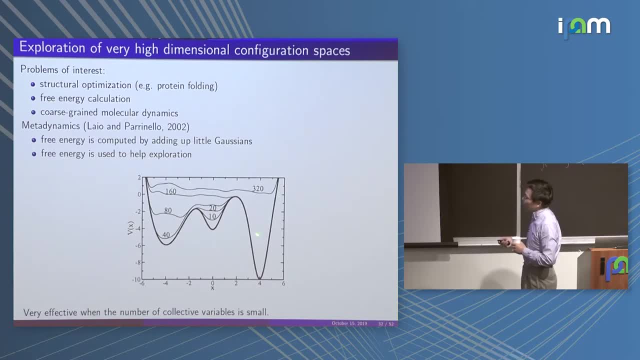 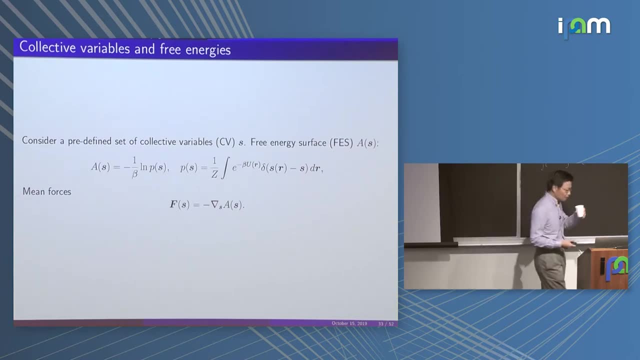 So here the objective is to compute the free energy. So let me maybe first say something about the free energy. You have this atomic system that we just talked about, but you don't want to track the dynamics of each atom. You want to look at a coarse-grained version of that. 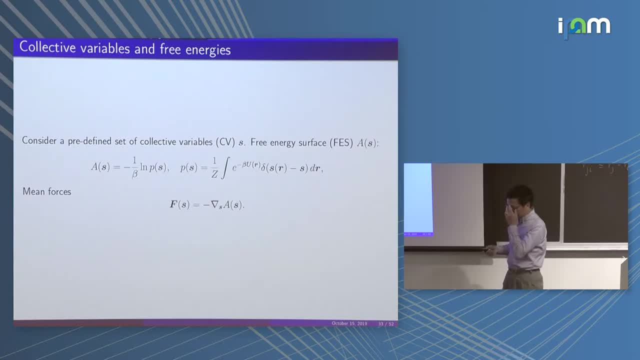 For example. that's typically the case. Okay, It's typically done in chemical engineering, where you have bees and springs. But how do you get the potential for that bees and spring system, whatever coarse-grained system, And how do you do coarse-grained molecular dynamics? 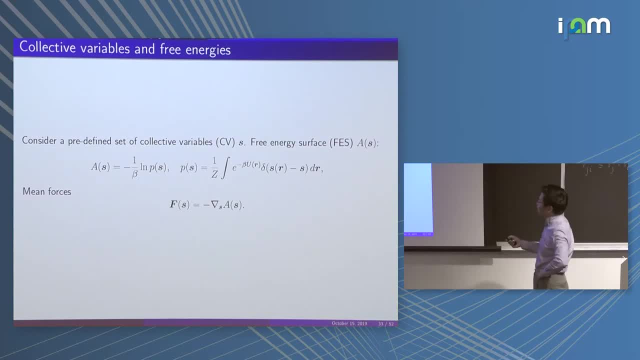 So this has been a difficult problem for a very long time. So let's just look at the free energy. So free energy is that you already predefined a set of collective variables. These are coarse-grained variables, For example, dihedral angles. 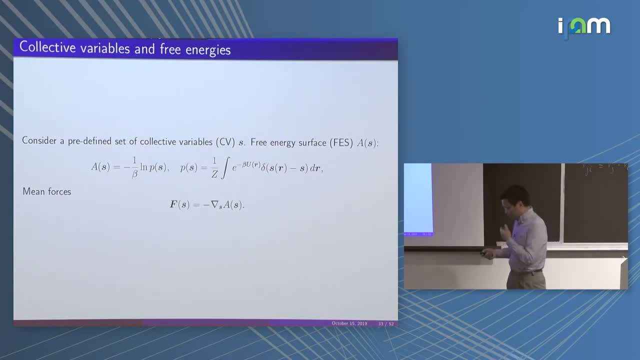 In a protein, Or these Steinhardt variables in a crystal, for example. So these are collective variables And you want to get the effective potential for that set of collective variables, And the effective potential is called the free energy. The free energy is different. 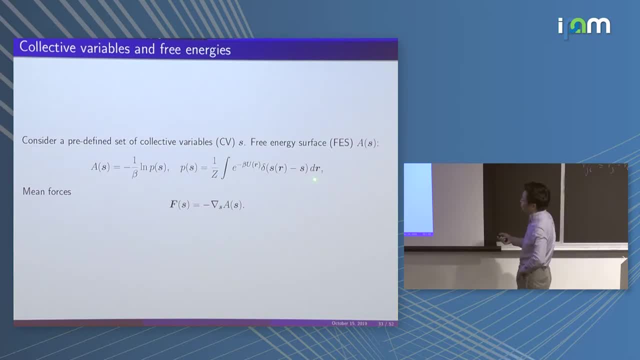 The free energy is defined in the following way: So you are integrating over all the microscopic variables. that has been coarse-grained, Essentially that's the idea. And then you have the mean force. So this is the sort of concept of free energy and mean force. 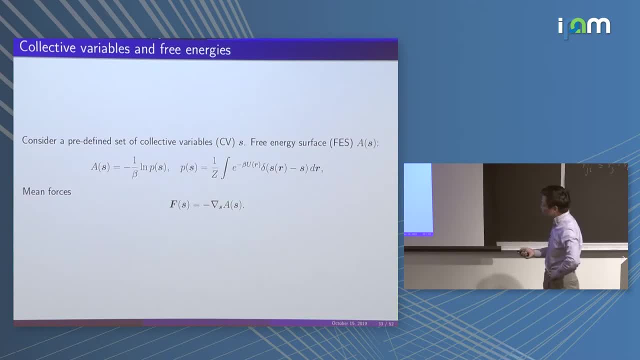 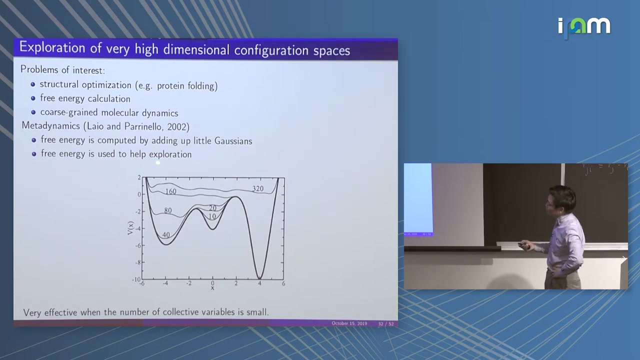 We want to get this free energy. So, in a way, this is the same problem as before. Before we had the potential energy, Now we have the free energy. So the issues are very much similar, Okay, Okay. So metadynamics, which is very well known, does the following: 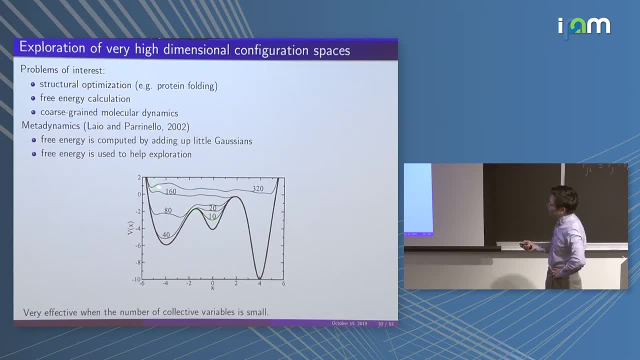 So the free energy is computed by. You are exploring this configurational space of the original configurational space. When you do that, and then you add this, At each point you add a little Gaussian, and that Gaussian is added to the correct. 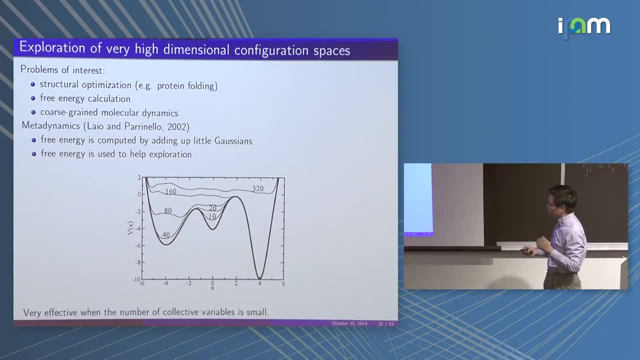 free energy, Coarse-grained variable, That of the coarse-grained variable, And then these little gaussians would add up to the free energy. So this is one idea. The second idea is that you are using the free energy that has computed. 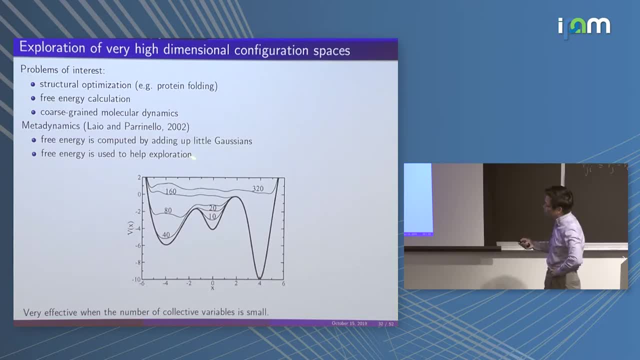 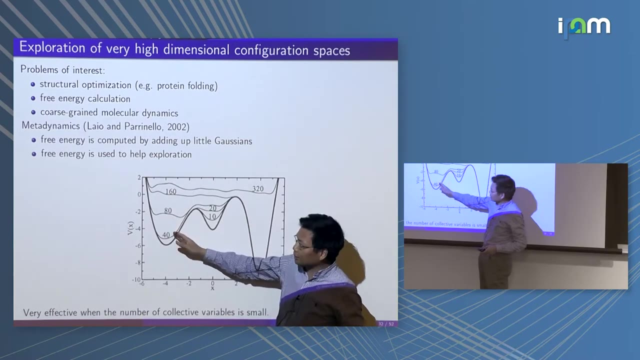 which is not accurate, but you still use that to help do exploration. So therefore you have a little. if you added a little Gaussian here, your potential energy doesn't look like this. it looks like this: So this bottom is raised up a little bit. so therefore you get less, get stuck. 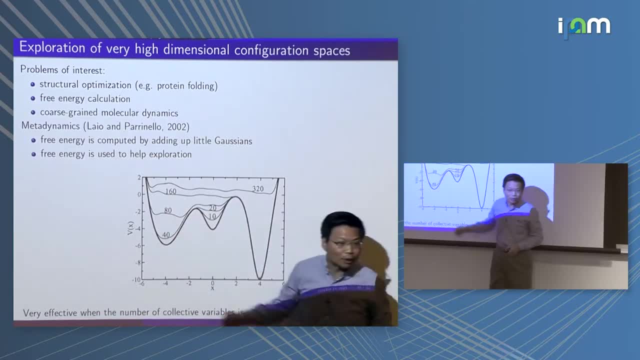 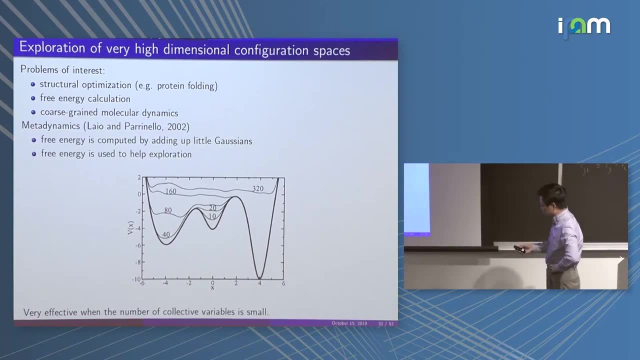 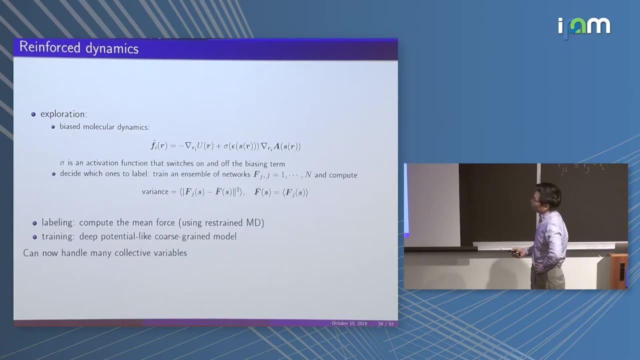 here. When you add up to here, then there's this: well is removed, so therefore you don't get stuck at this well at all. So this is the idea of metadynamics, And this is a little bit like what I was emphasizing about exploration. Okay, so now we could cut something called reinforced dynamics. 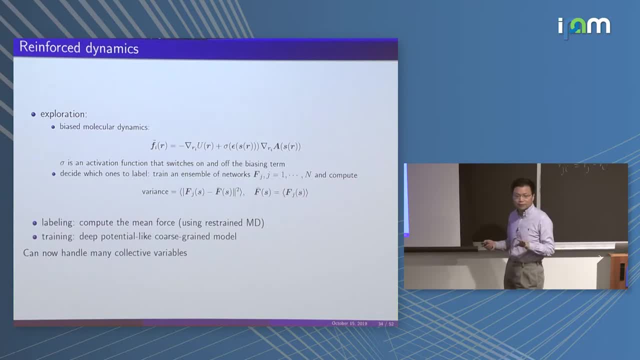 Okay, so now we could cut something called reinforced dynamics. Okay, so now we could cut something called reinforced dynamics. We call it reinforced dynamics because there's an analogy with reinforcement learning, but that's not the point I wanna make here. So this again has three parts. 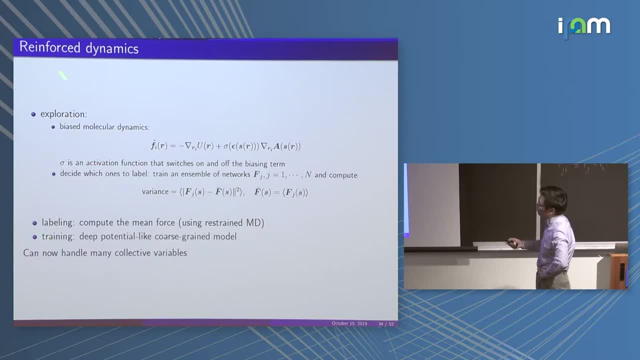 exploration, labeling and training. And the part about exploration is the following: that you are exploring with a modified potential energy by adding this part. So this is a little bit like the metadynamics, except that there's a sigma here. So A is the field of energy you computed so far. 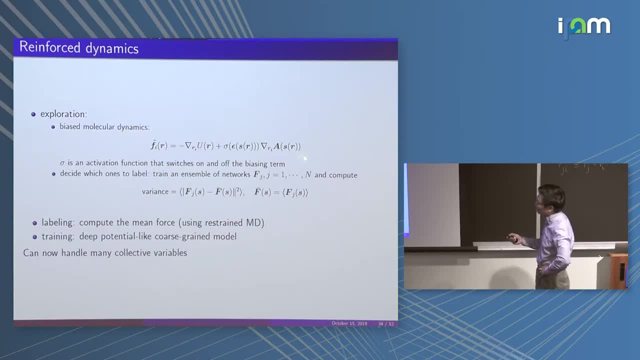 which is not necessarily accurate. Because it's not necessarily accurate, we're gonna switch on and off of this biasing part depending on how confident we are about the accuracy. So this sigma here is a sort of activation function which activates this term. 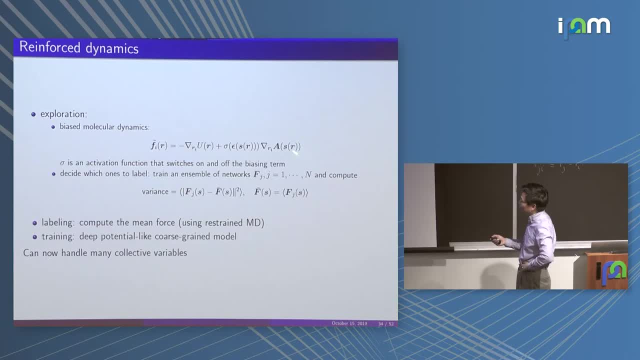 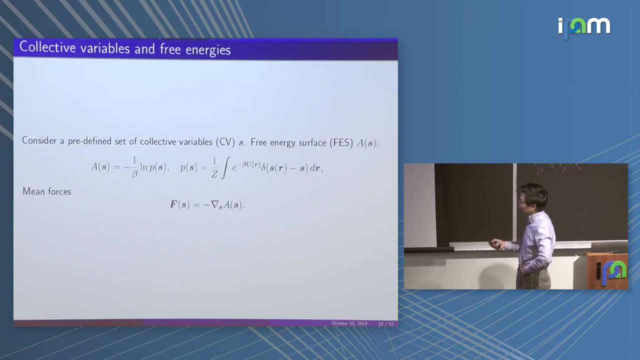 If we are very confident, very confident, very comfortable about it, very confident about it. if we are not so confident, we just switch that off. So you should notice that, because we are not doing these little gaussians, we're doing a neural network model. 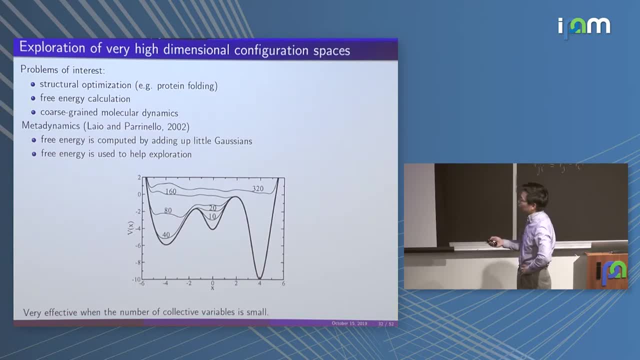 so that's more global. So that term is important to switch on and off. If you're here and you got something really wrong and you still use that as a biasing, that wouldn't be good. Okay so, and then? 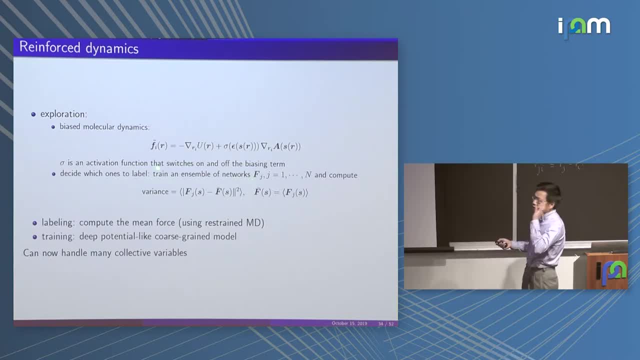 you know, once you see a configuration and you need to decide whether you need to have that label, namely compute the potential mean force in order to compute the free energy- And that decision is done by this little trick I mentioned earlier, namely having an ensemble of networks. 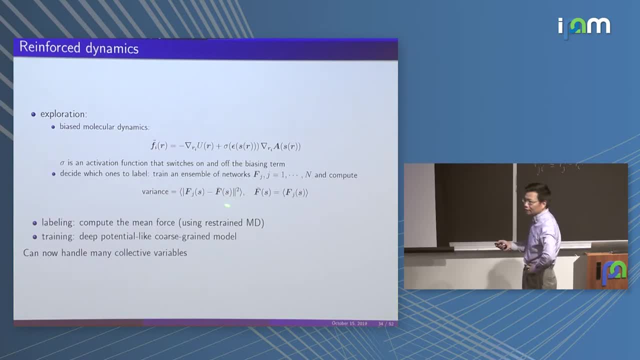 and compute the variance of their predictions. If the variance is big, you have that labeled. if it's small, you don't have that labeled And labeling is done. so labeling: you need to compute the potential mean for potential mean force. 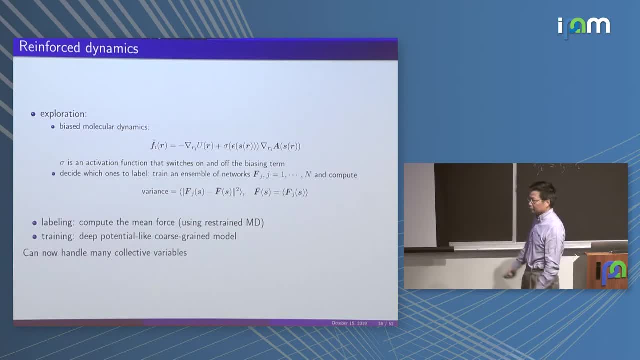 And that's done by restraining. we'll look at that in a second. Yes, So when you compute the variance here, some of the data will be coming from a biased sampling right when the activation function has been switched on. Yeah, 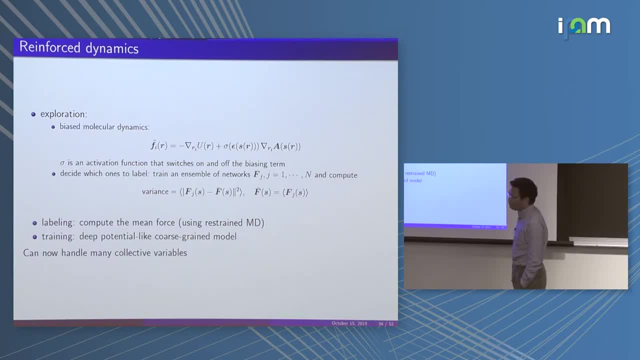 Are you going to revate the variance to take that into account? Pardon me, The variance that you're-. Oh, the variance. no, The variance is just whatever you've computed, But it has been, it could have, so it's been computed. 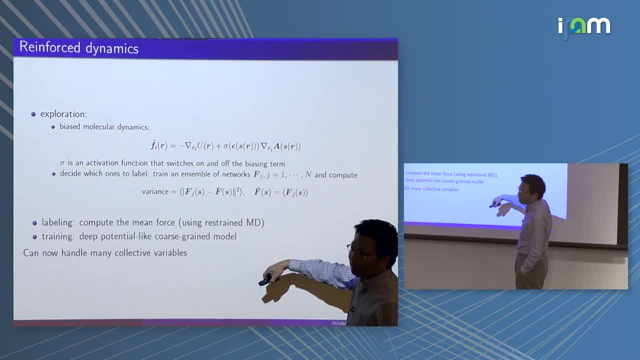 it's being computed under the effect of a biased ensemble. Yeah, Is that really fair? Because you would have liked to look. that could be misleading, for example, that could be systemating. Don't you think that would be a systematic effect? 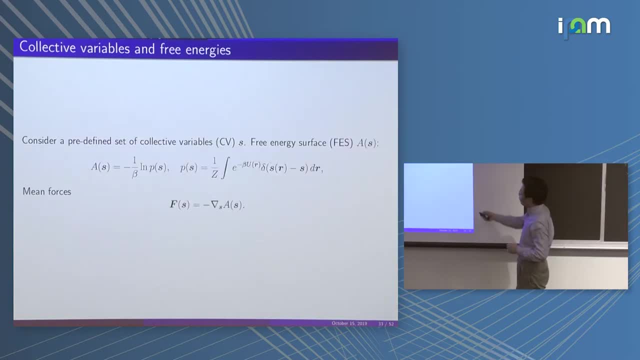 No, I'm just trying to compute that. I just need to compute this integral right. As long as I have enough terms in this integral, I'm fine, Fair enough. but I'm comparing with the previous one, the interactive potential. 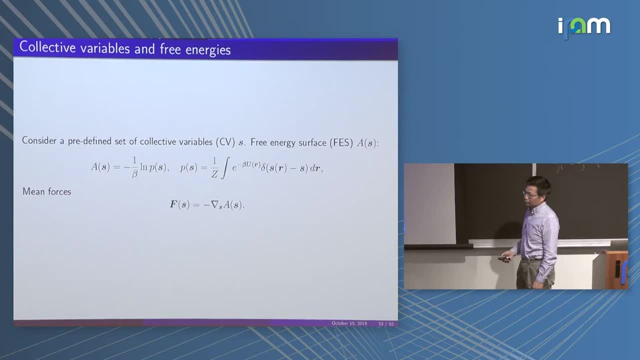 Yeah, When you computed the variance, the data was inherent. right, The variance is a bias. No, the variance is the variance between the different neural networks. I'm training five neural networks on the fly, not just one, And the variance is just between the five neural networks. 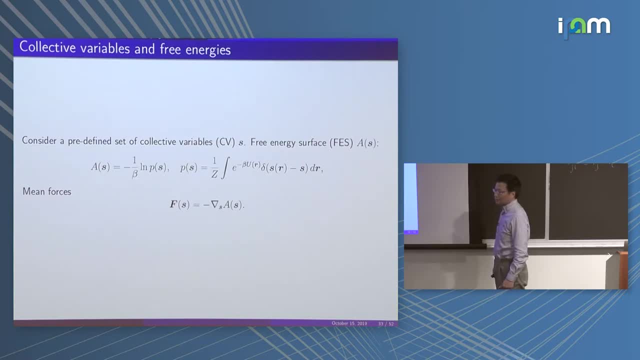 Yes, but it's. is it a Boltzmann weighted variance? No, no, just the straightforward variance. I'm just comparing five numbers, You know. if they're all the same, I'm good and it's happy, so don't do any labeling. 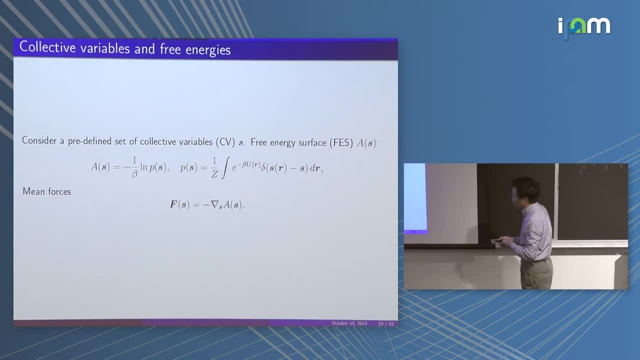 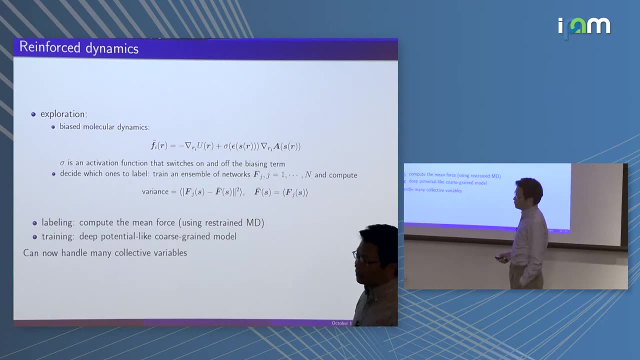 If they're all over the place, then label that. Yes, So you said that sigma is switched on and off depending on the accuracy of A. but is it the accuracy of A or the accuracy of the gradient of A? Because they they can be very different. 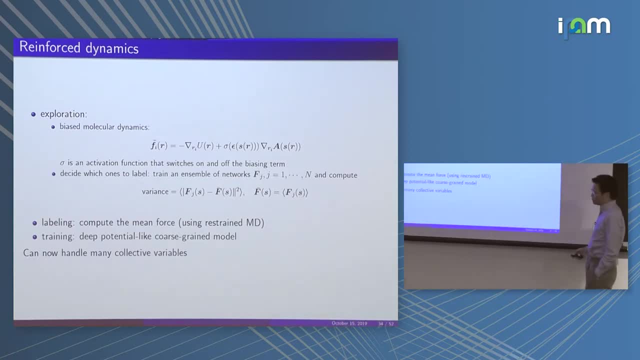 Gradient. Oh, I see, yes, Okay. so the advantage of of this kind of ideas compared with meta-dynamics Is that now we can work with many collective variables. So many meta-dynamics is limited to, you know, less than 10 collective variables. 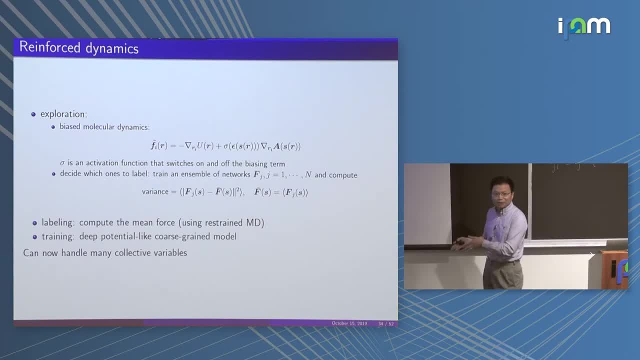 So in that case you really have to make sure your collective variables are really the right collective variables. If you want to look at some sort of interaction and the collective variables is not the right reaction coordinate, and then you're, then you're really in serious trouble. 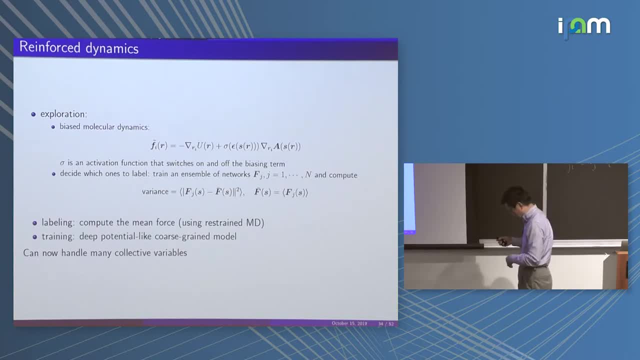 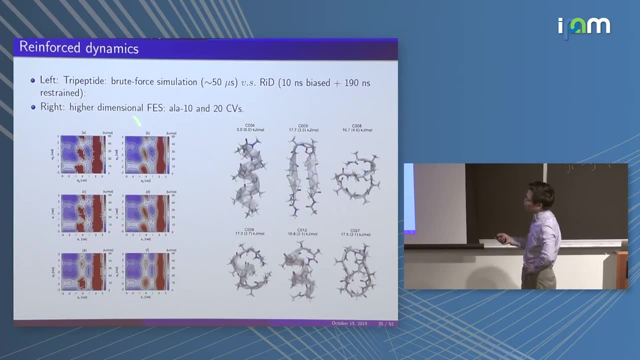 So now we can handle many collective variables. so we can. we don't have to be careful with so careful with the choice of the collective variables. So, for example, this is a trivial system: try a peptide And okay. so, and I forgot what was coarse grain here. 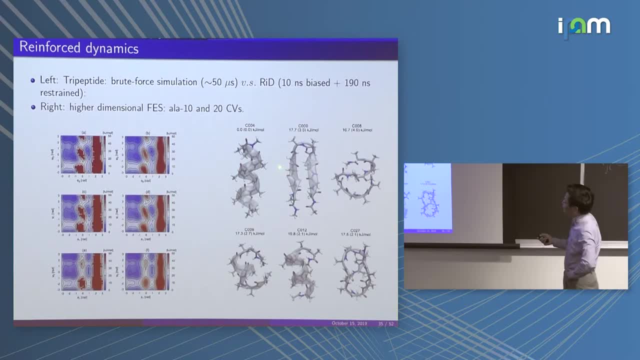 Okay, anyway, try peptide. So this is a mathematician's version of a protein Namely. you put 10 or 11 alanine, I think, And then yeah, alanine 10, with 20 collective variables. 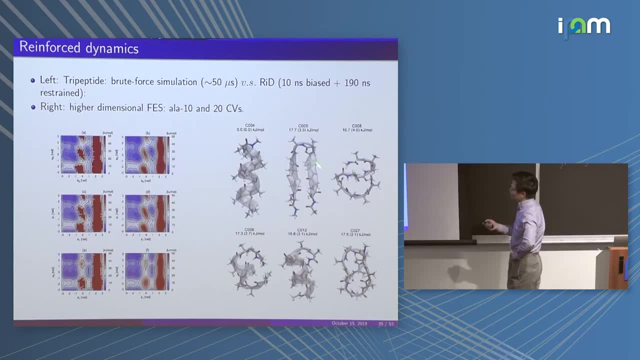 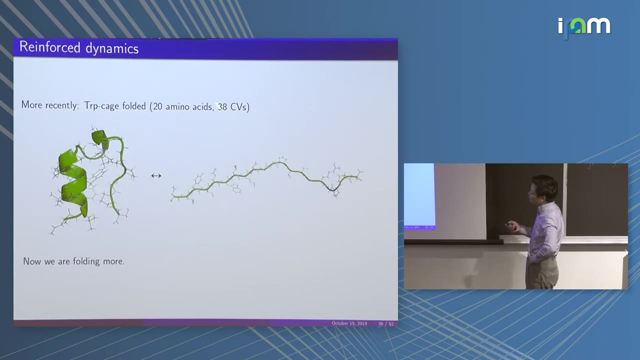 so the two dihedral angles, phi and psi, And this is a 20-dimensional configuration space and you can look at, enumerate all the metastable states Now and you can use that to fold proteins. This is a little protein with 20 amino acids. there's 38,. 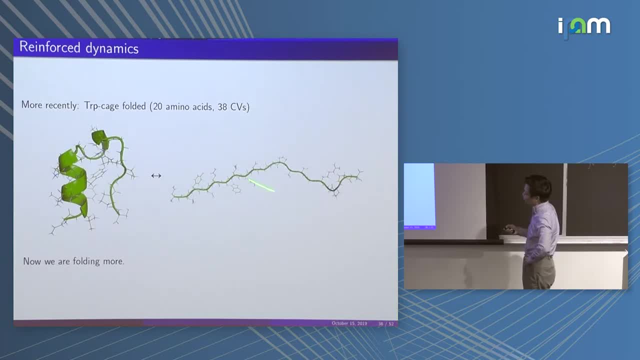 collective variables. This is the initial configuration and this is the folded structure, So we haven't really worked very hard on this, but I think, if you do, you can do this with hundreds of collective variables, And this really opens up a lot of possibilities. 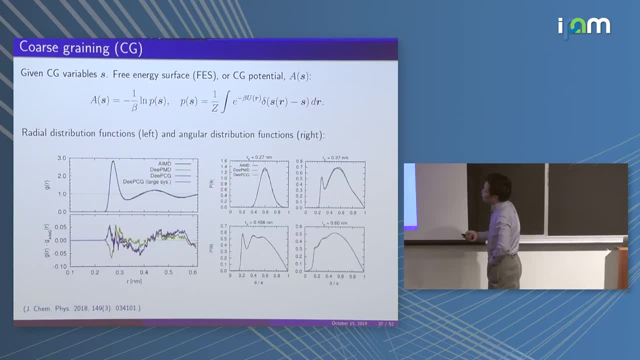 But we haven't really worked very hard on this. So this: with this you can now do coarse grain. molecular dynamics: Yes, When you're using the variance, you select the examples to label: Yeah, Are you selecting one example at a time? 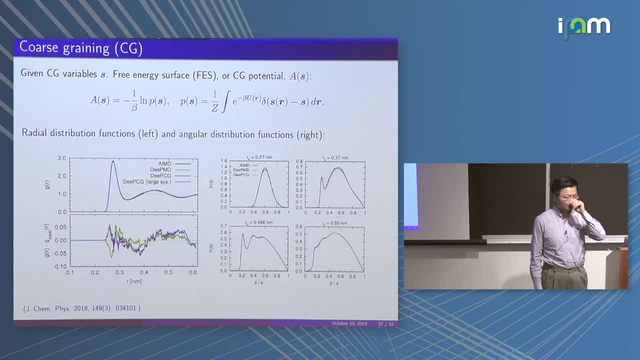 or are you selecting many examples? No, just that particular configuration, But then you label it and then you re-compute the variance. so you're doing one at a time selection, or do you do? Yeah, you do the loop, you do the whole loop. 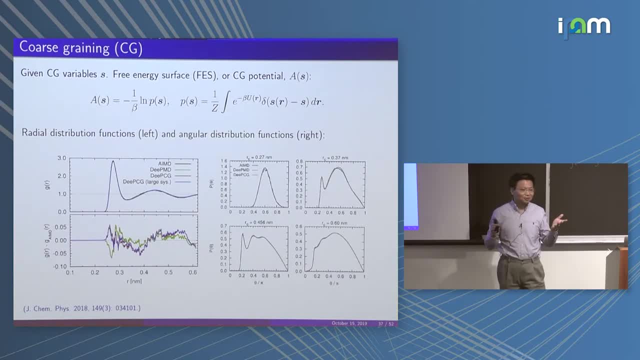 Right, but it's one at a time. You don't have a batch, Okay, so that can be debated. right, That's a little, that's some. Maybe you label it and you don't train with each new label added. 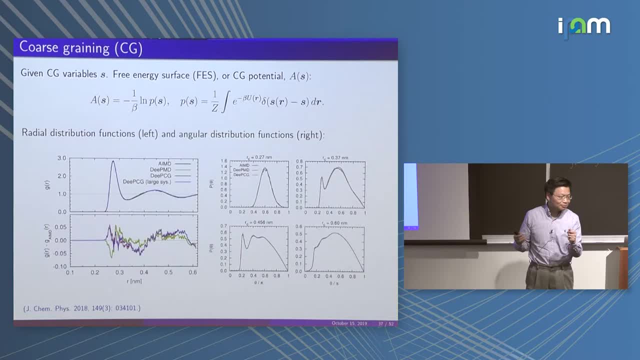 You can wait for a little batch and then retrain, But then you have a covariance problem with the variances. That could be, yes, that could be. So certainly there's a lot of algorithmic issues one could think about. So when you collect the data, 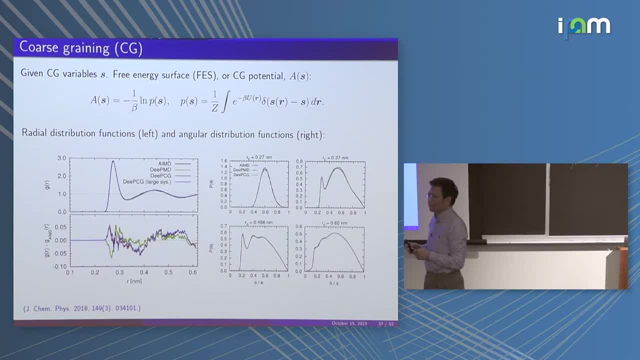 you start the whole bunch of molecular dynamics at batch configuration. You do the restraining- So suppose this is the collective variable that we want to label- and you do sort of a restrained molecular dynamics, to make sure I'm really sampling with the correct Yeah. 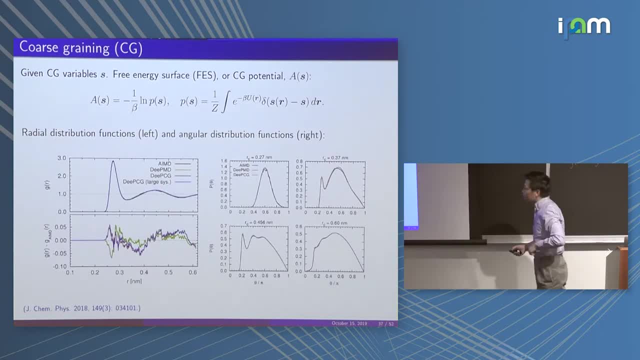 Yeah, So then you can do coarse-grained MD Anyway. so this is a coarse-grained MD with- I think it's also for water- Then you can see that you know you really got this kind of very good accuracy by the standards of coarse-grained MD. 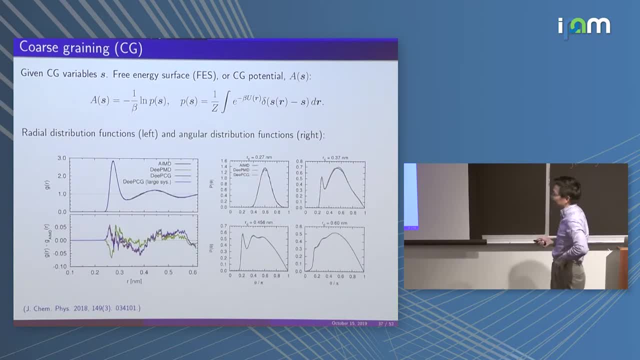 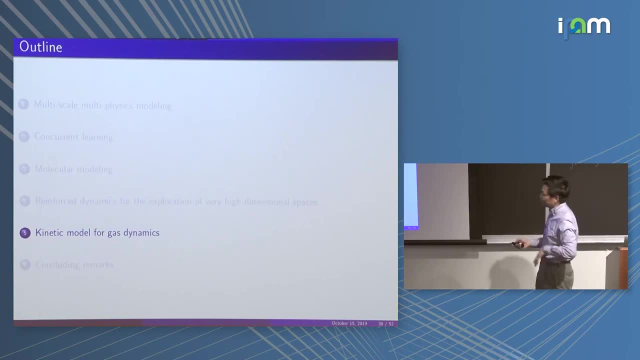 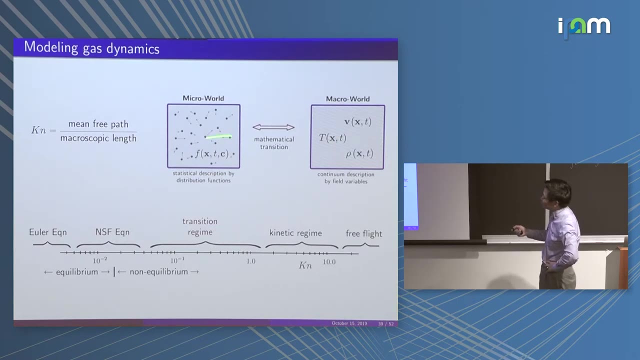 So if you really have to read the literature of coarse-grained MD to appreciate that this is good accuracy, Okay, so the last example is a kinetic model for gas dynamics. So this is gas dynamics, The important quantity. you know, these are gases. 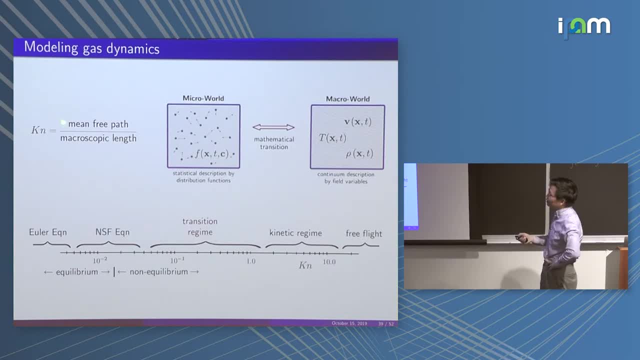 Gas and molecules collide with each other. An important quantity is the Newton number, which is the mean free path, That's, you know, the path between collisions and the macroscopic system size. So that's a Newton number. If the Newton number is very small, 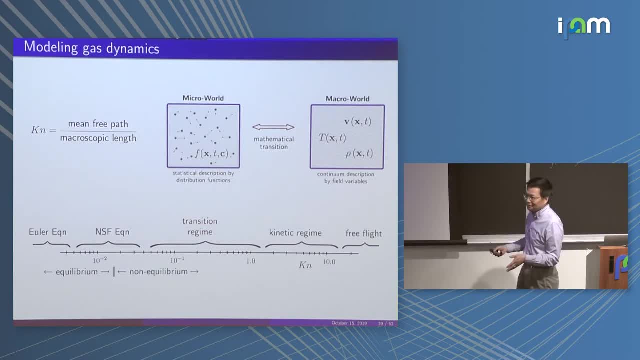 how big is the Newton number in this room? Does anybody know? Okay, I don't know, but I don't know. But it's supposed to be small, because here we're supposed to be able to use Euler's equation. So then we're just looking at density. 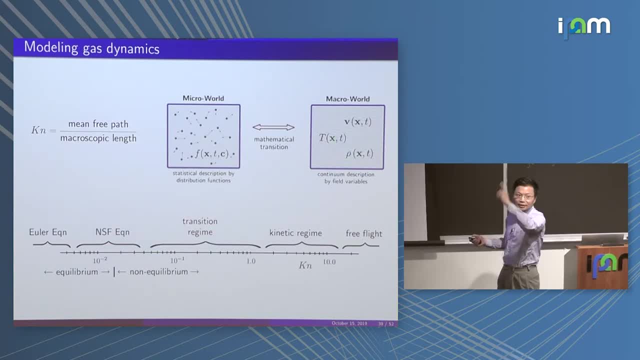 velocity and temperature. And if you're up there, you know, in the sky the Newton number could be very big. then you really have to use look at the collision of the atoms and use Boltzmann equation. And if you're designing for shuttle, 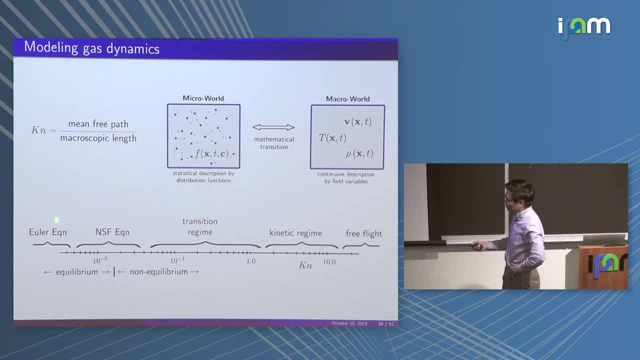 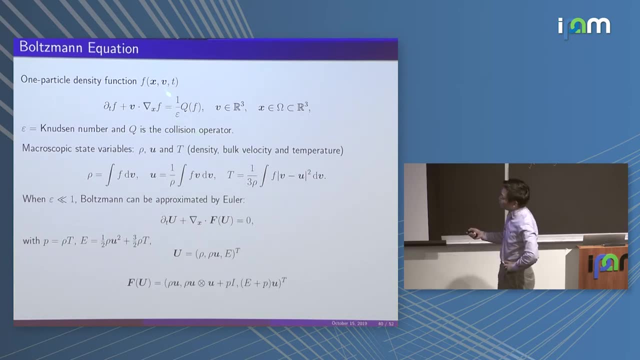 and then you have to look at the, the whole regime, when with a small and large Newton number. So the Boltzmann equation looks like this: where you have this Newton number- here epsilon is not necessarily small- and you have the collision term. 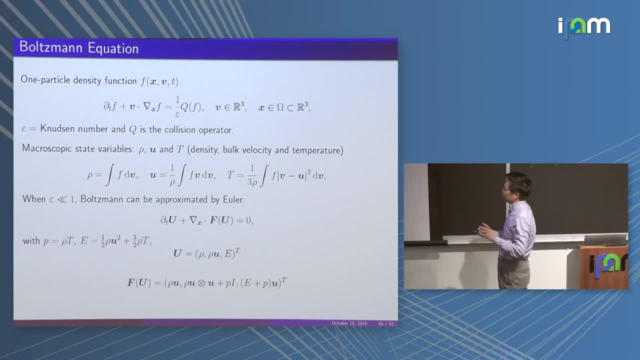 and the collision term is a rather complicated integral operator. So this is the Boltzmann equation, And Euler's equation is obtained when you take in the epsilon going to zero limit. In that case, we just have to look at these, you know. 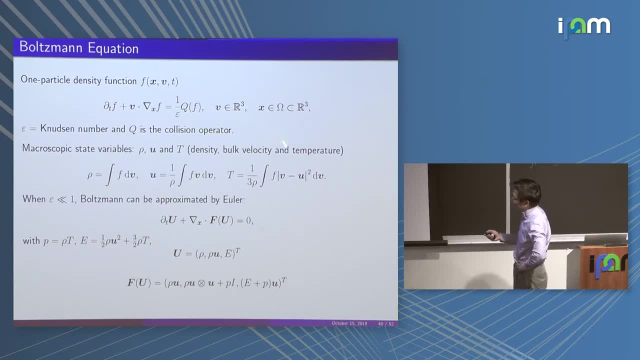 we just have to look at these zeros order, first order and second order moments, trace of the second order moments of that distribution function. So F is the phase-based distribution function. So we get a closed system for these low order moments and that's Euler's equation. 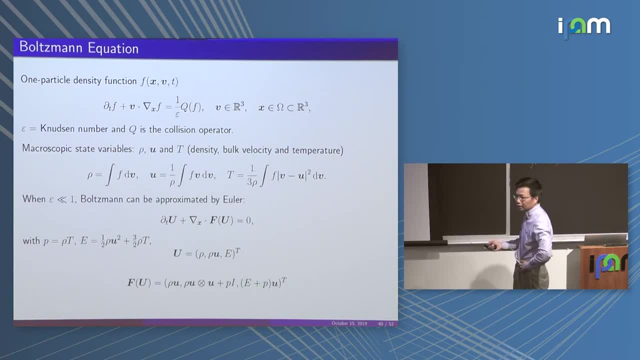 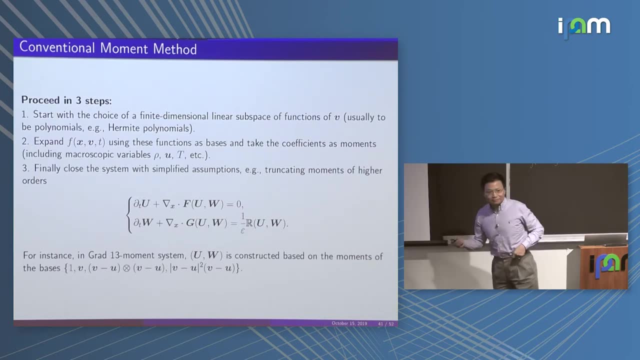 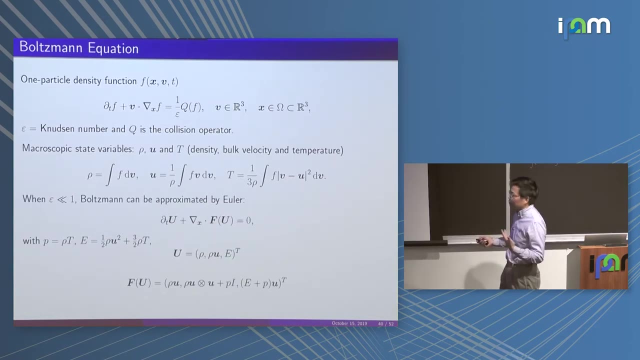 And this looks like this For ideal gas. this is how Euler's equation look like. This is great for epsilon small. Now people have thought for a long time about extending this set of ideas to large values of epsilon. So this is the moment. closure problem. 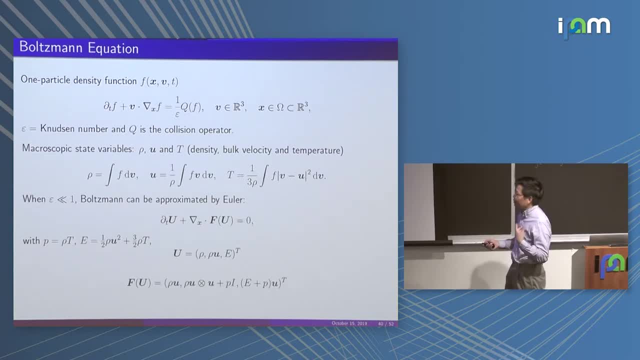 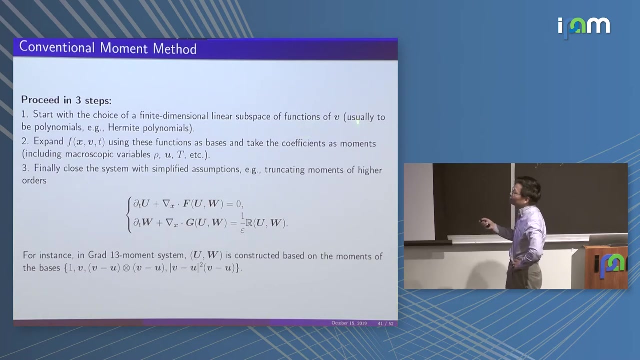 Start, as far as I know, it started from a hired grad at Quran Institute in the 1940s. So here is the idea Basically. you want to extend this to more moments, So you started with finite dimensional linear space of functions, polynomials usually of V. 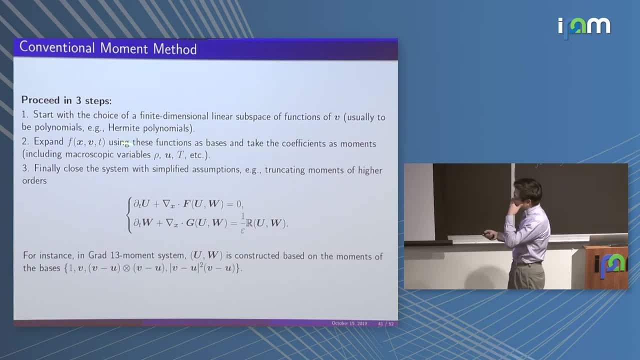 So these are generalized moments, permitted polynomials usually, And you expand the function using these spaces And then, with this expansion, in the end you have a closure problem. As always, you have a closure problem because the equation of low moments involves higher moments. 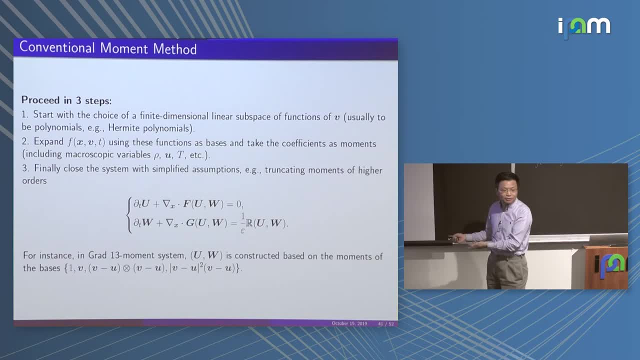 higher moments, even higher moments, and at some point you have to close off that thing, that hierarchy. So this is the closure problem And then just truncate it, usually at higher orders. So this is the moment closure scheme that has been. 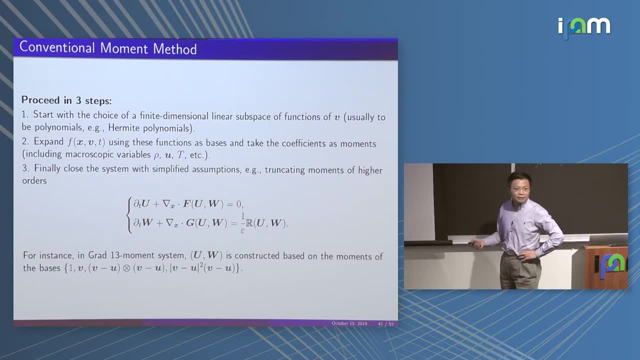 that's been done. It's been pursued for a very long time. The problem with this is that there are two problems. One is that the equation you obtained is not necessarily hyperbolic. For example, grad's 13-moment system is not hyperbolic. 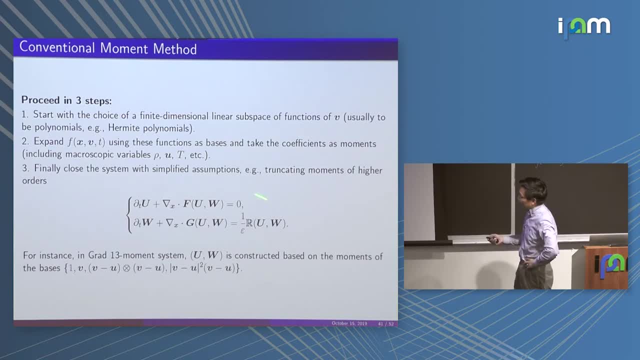 at some of these places. And secondly, that the accuracy is not guaranteed. because you did this closure by truncating or by something else, You know there's no guarantee of the accuracy. So now we know that we want to do this with machine learning. 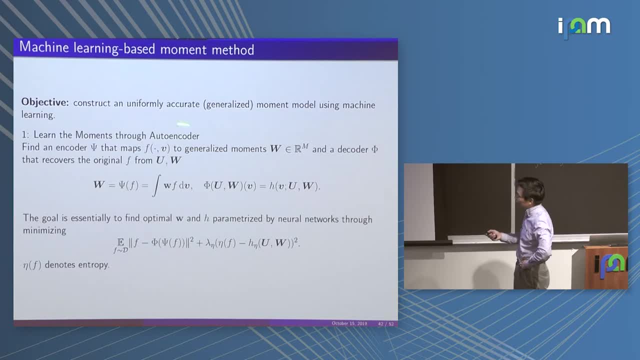 What else do we do right? So we do this in two steps. The first is to learn the moments through an autoencoder. Okay, So here you want to find the optimal set of w so that, so that, once you get, so that the moments, 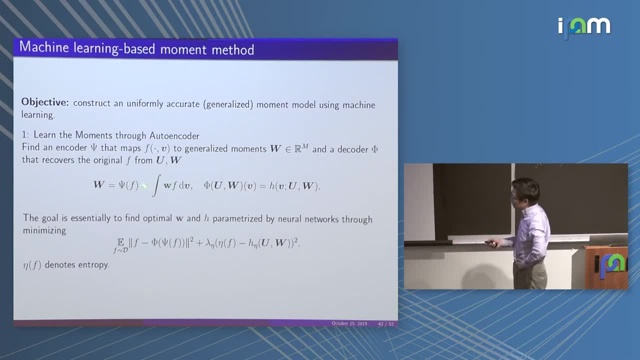 so w is not a general function, not necessarily polynomials anymore, So so that the generalized moments created by this w function best represents the original distribution, the original distribution function. In other words, if you reconstruct the original distribution function using only w. 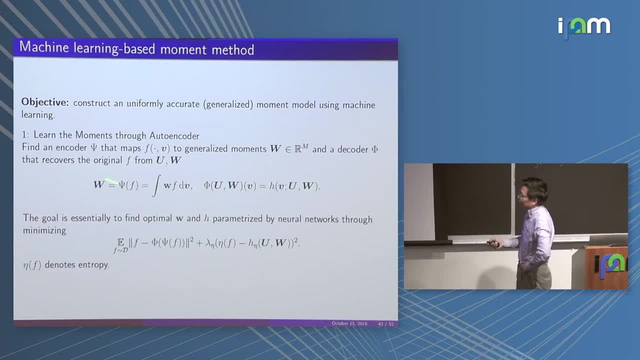 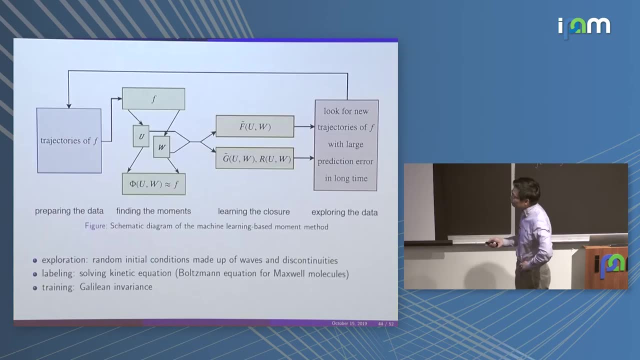 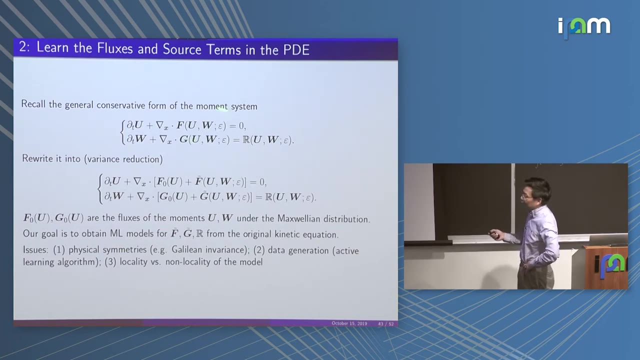 the accuracy is maximized. So this is how we generate generalized moments. And then, once you decide what these generalized moments are, boy, what? yeah, once you decide what, you then try to get the dynamo equation for the generalized moments. 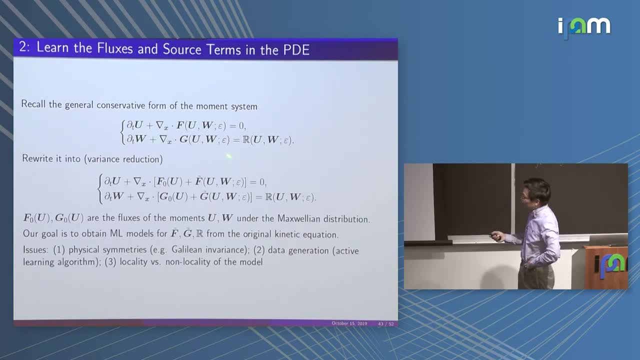 Well, this is the w, the new moments. This is the old one. You have these fluxes and source terms. For some reason, empirically, we've found that it's much better to do this. Namely, you should take into account the Euler part. 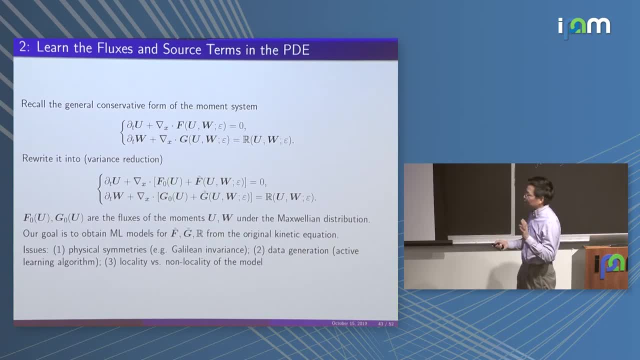 The Euler part corresponds to the local max w, that the distribution function is close to local max w. And then do this. This seems to be a very good variance reduction algorithm. Now, the data you want to generate are kind of noisy, and by doing so the variance is greatly reduced. 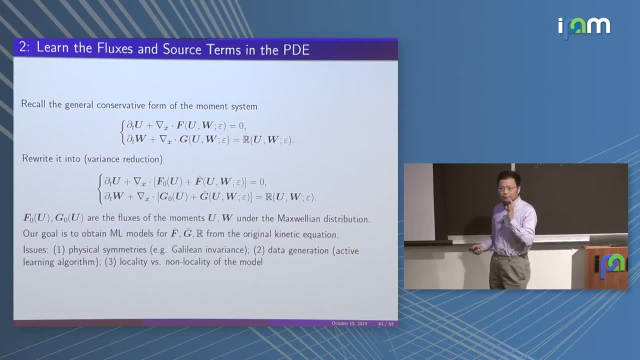 So what are the issues? Well, again, symmetry is important. So, since now we're looking at a dynamical problem, before, when we did the functions, those were static problems. So the symmetries are, you know, the usual symmetries. 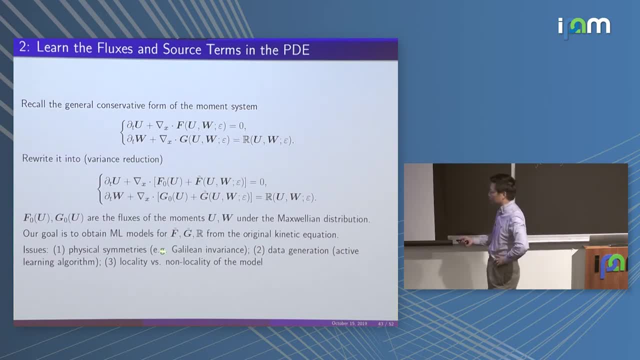 This is a dynamic problem, So there's one, at least one additional symmetry, which is the Galilean variance. So that's one issue. Secondly, how do we generate the data? Thirdly, how do you, if you want these models to be really like your PDEs? 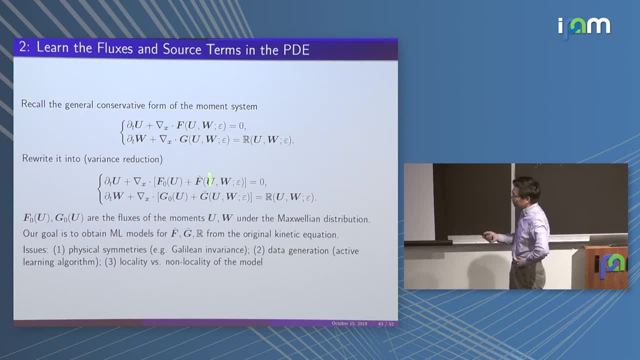 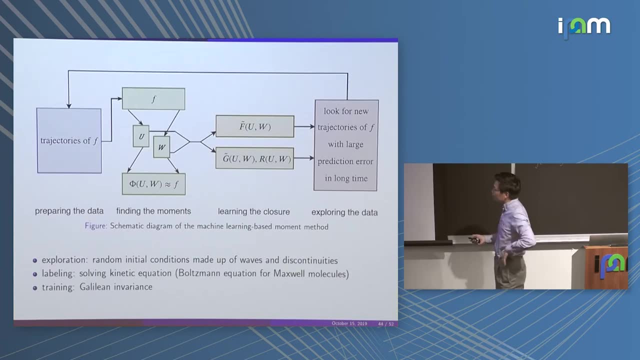 not just in the algorithm. how do you select the training algorithm, the neural network model, local versus non-local? Okay, so this is the whole procedure, which is just the same as before: active, what is called concurrent learning, and now exploration. 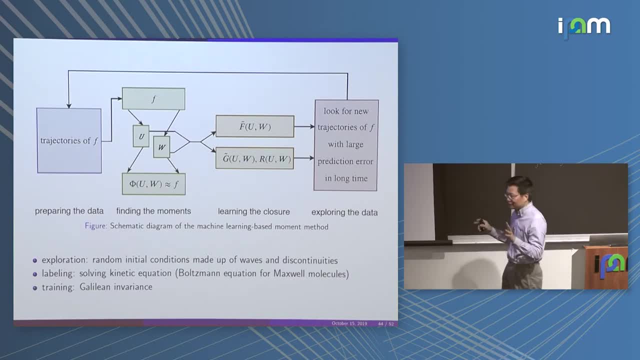 So this is a poor man's exploration. I want to emphasize: how do we do exploration here in the best way? It's not. it's clear. So this is a poor man's exploration. What do we do? We cook up a set of random initial conditions. 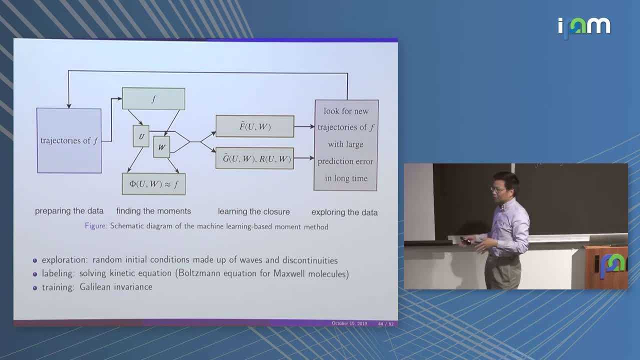 That are made up of waves, random waves, separated by shocks, Because this problem we have to deal with. shocks Okay, And labeling is just solve the kinetic equation, ultimate equation, And then the training part, as I said, we have to take into account. 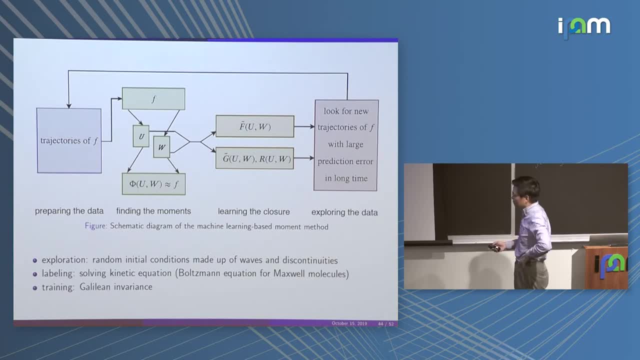 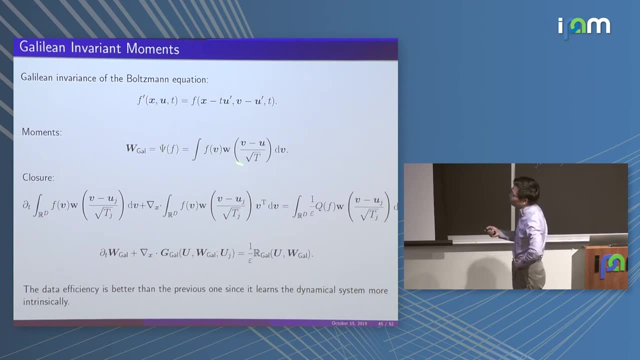 besides the usual invariance and conservation laws, we have to take it on the Galilean variance. Okay, this is just to give an example how to do Galilean variance. We choose the moments to these functions w to look like this: 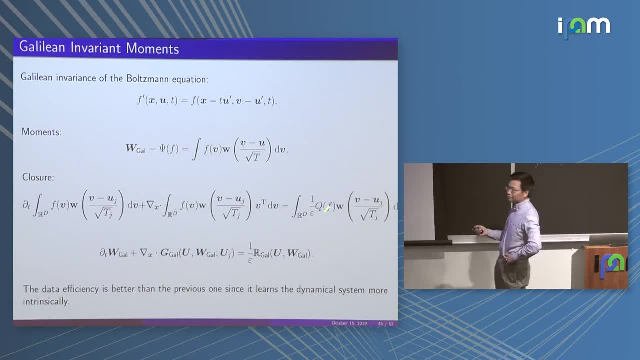 This removes the Galilean variance And then everything works out. This is a simple idea, trivial idea. you could say that we took a long time to figure out that this is important. So if you don't do this, then you need lots of data. 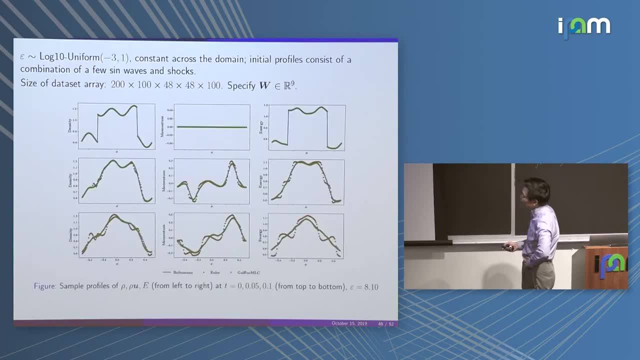 If you do this, the data needed is greatly reduced. Show you some results. This is: we take the Newton number to be random variable selected from this distribution: log distribution, log, normal distribution, log, uniform distribution, And then this is from 10 to the minus one to 10 to the three. 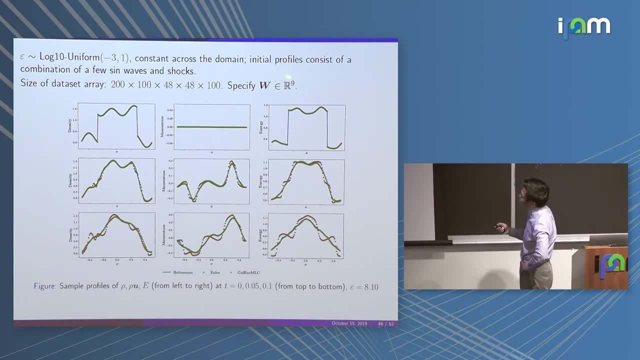 or something like that. And then we, for the additional generalized moments, we select nine. Again, this is sort of done by hand. And then for the microscopy model, the bottom equation, we use the model with Maxwell molecules, By the way, even though there's been a long time. 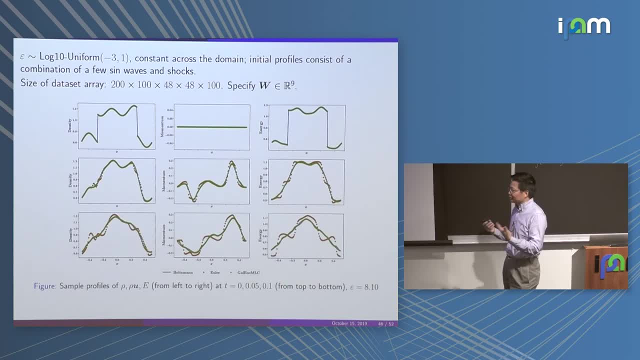 where people look at moment closure. it seems that there's not a single moment closure created for realistic models, namely Maxwell molecule that doesn't even exist. We try to compare with existing models. couldn't find. So these would be results of density. I think density. 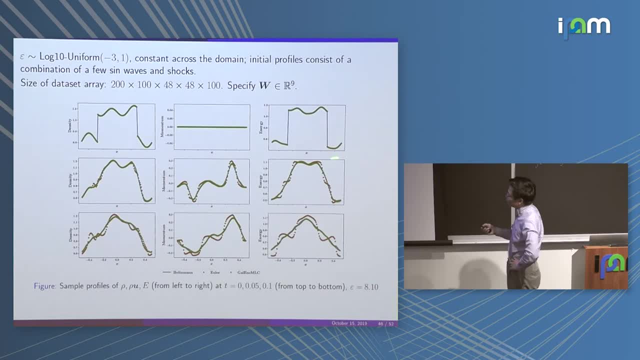 what is it? energy momentum density at initial condition, later time, even later time. and then the green. there's three curves here. This orange curve is just if you solve all the equation and you know it's not gonna be very good. 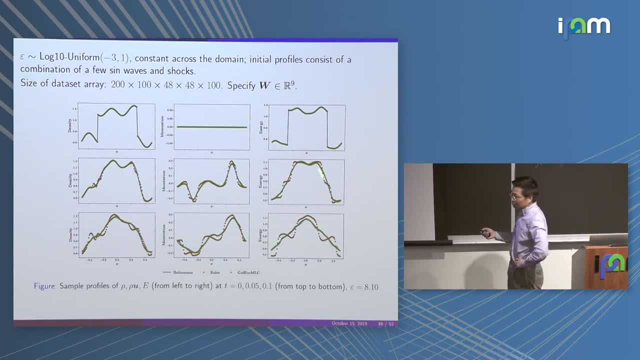 And then the green curve. green curve is solving the moment generated the machine learning-based model. The epsilon value here is 8.10, not small, or 8.1, not small. And then there's a blue curve. 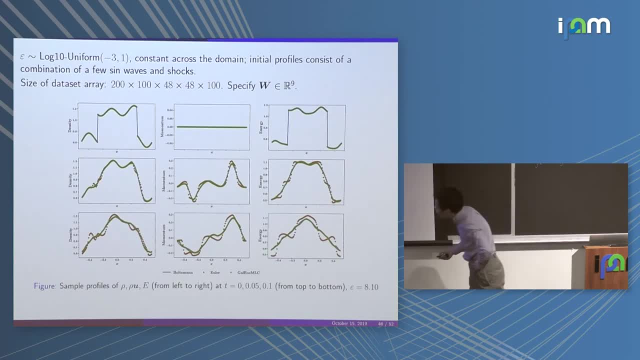 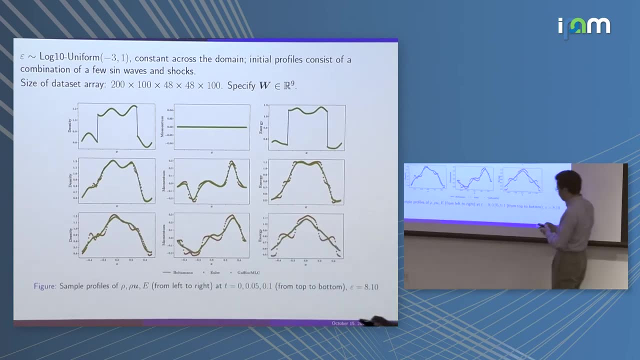 which is the solution to the Boltzmann equation. You don't see much of a difference, because in this particular example actually there is a difference. here There's blue and green, that you see. But overall this is a typical example that we've seen. 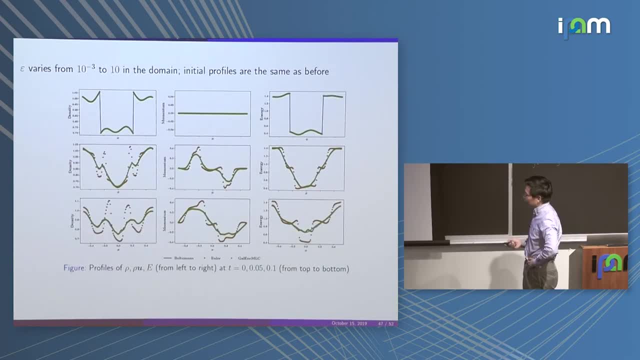 Overall, the accuracy is very good. Another example: same thing, but this time the epsilon changes across the domain just to mimic transitional regime. So this is the results. this is how the generalized moments look like for a different set of, so they're not polynomials. 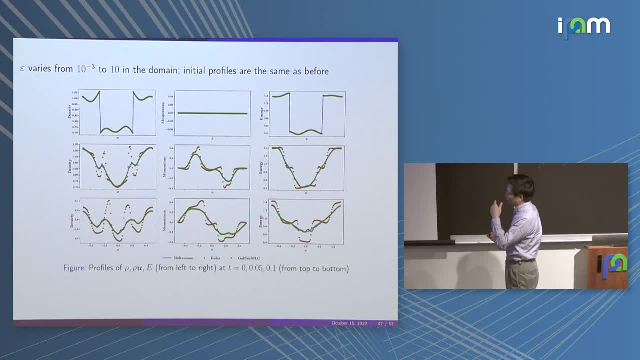 So this is part of the. the problem is not as complete as the one we did before, So there's a lot of work to be done in order to make this really practical and for everybody to be able to use. There's still a lot of work that needs to be done. 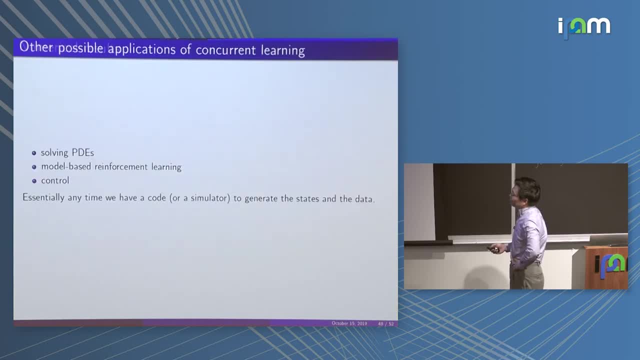 Pavement just got accepted. So to conclude, there are other possibilities of concurrent learning. For example, if you want to solve PDEs, you have a PDEs in front of you, having the Jacobi-Bellman equation. There's no data beforehand, and then you need, you can. 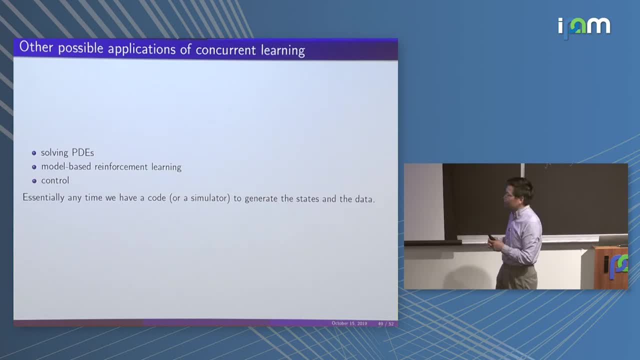 cook up this kind of concurrent learning procedure to generate the data and learn at the same time interactively. Model-based reinforcement learning. Here model-based means really model-based Reinforcement learning. when they say model-based, typically it's model-free. 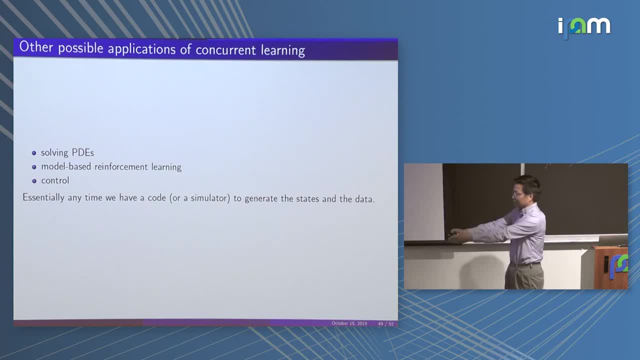 but they're also talking about model-based. But what they mean is that they first learn a model and then use the model-based. But here, when I say model-based, if you, you know, if you have some dynamical system in front of you, in front of you. 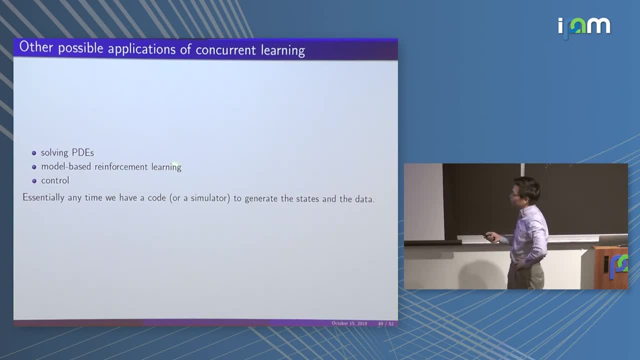 and you really can use that details of dynamical system to do reinforcement learning. And again, this is a problem that starts out with no data And this interactive process should be helpful, especially when the model is sort of reasonably complicated, So exploration is not. 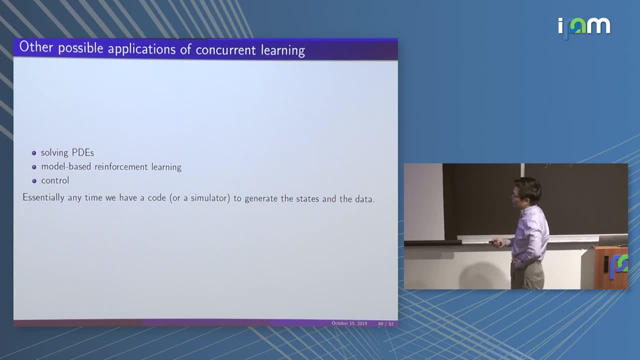 exploring the state space is not so easy. Okay, essentially, anytime you have a code or simulator to generate the states and data, you can use this concurrent coupling. Concluded remarks: Concluded learning is a very powerful tool. DBM data: okay, I already said these. 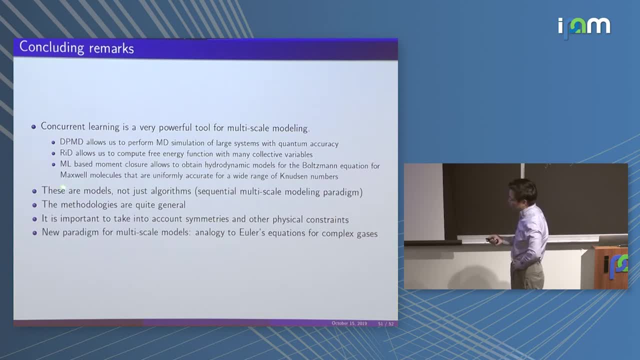 but I want to say that these are models, not just algorithms, but these models can then be used to do sequential multi-scan learning. So these are concurrent learning, but then sequential multi-scan models- Please get this straight- And the methodologies are quite general. 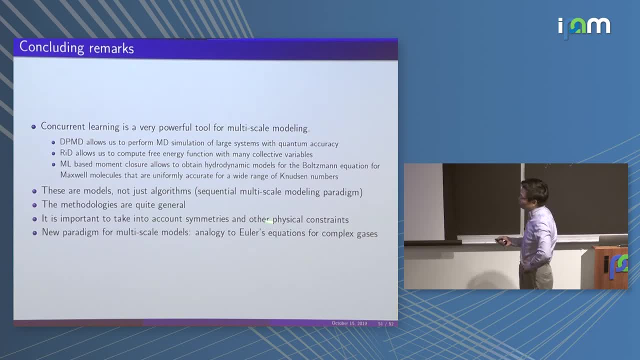 and it's important to take it on symmetries and physical constraints, And so how do we think about these models, which part of it is the neural network? So this is the example that I didn't know when I was a graduate student here. 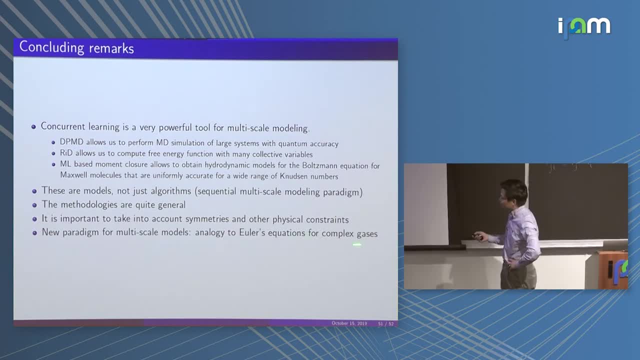 when we had to solve all the equations with complex gases. The equation of state is not just ideal gas, And in that case the equation of state, if I remember correctly, is stored as a table in Los Alamos. So here is the same thing. 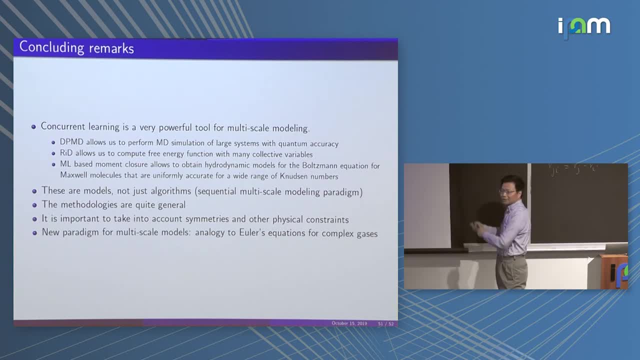 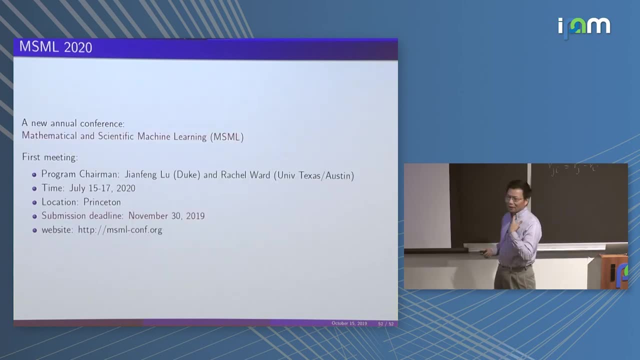 You have the equation and part of it is stored in a table somewhere, Basically, but you can think of it as just as a PD. I think that's important. Okay, This is my advertising slide. So we are starting a new conference. 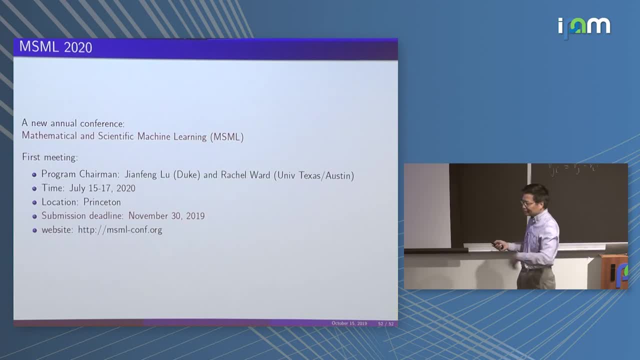 This is called Mathematical and Scientific Machine Learning. Stan and I are in the scientific board And the first conference is going to be Princeton, organized by two Princeton alumni, Jianfeng Lu and Rachel Ward. Going to be happening next summer And this is the most important part. 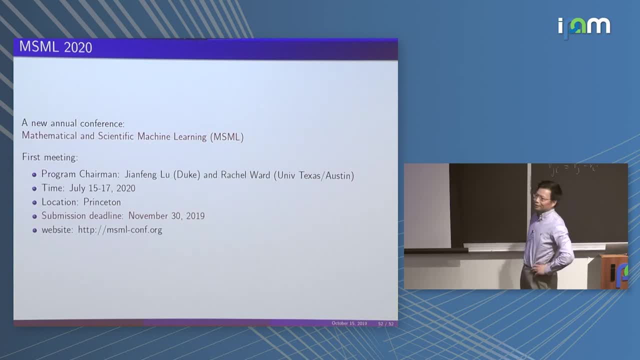 If you have a good paper, please submit before November 30th. That's all I want to say. Thank you, Thank you.